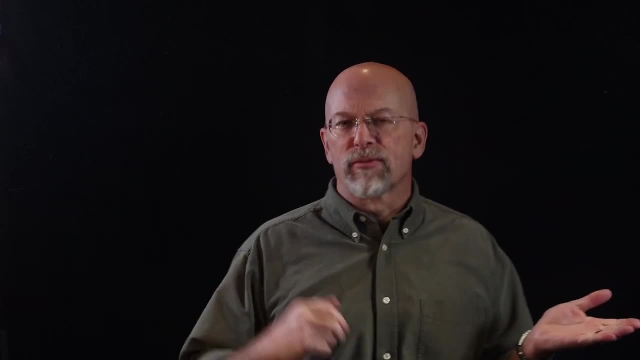 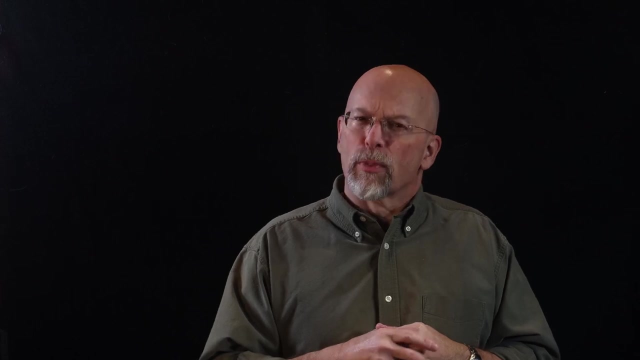 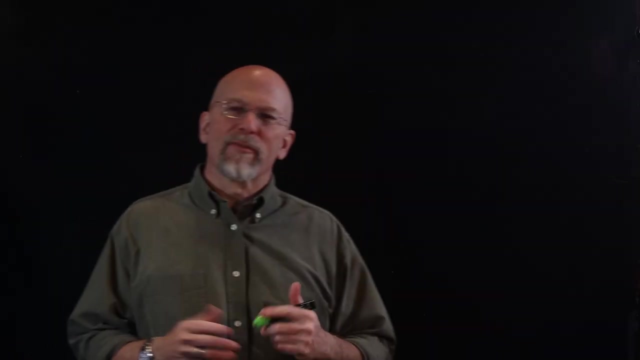 If you are comfortable with the concepts of a non-deterministic versus a deterministic finite automata, but are not comfortable converting from one to the other, maybe we can clear things up with a quick example. A couple of episodes ago, we presented a non-deterministic finite automata that was 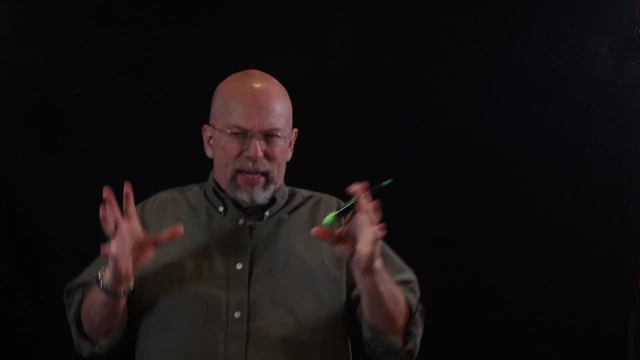 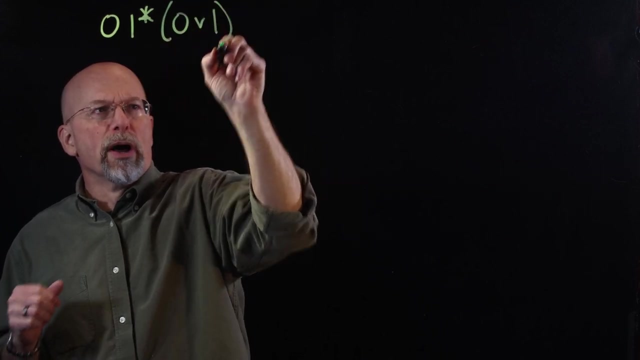 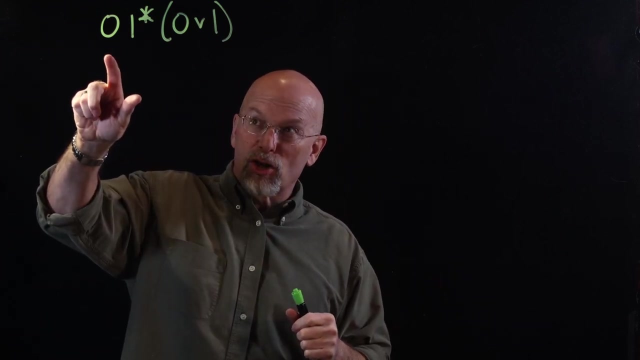 supposed to detect from the binary alphabet the regular expression. let's say 0,, 1 star 0 or 1.. All right, And so the regular set that was generated from that regular expression: every element had to start with a 0. And then there could be any number of 1s between that 0. 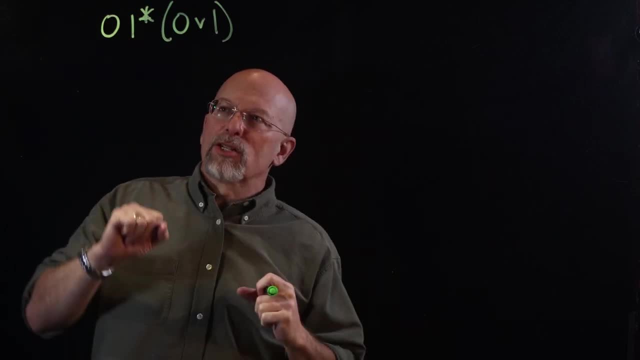 and a final 0 or 1.. Items that might have been in this regular set would be anything that starts with a 0. And then there could be any number of 1s between that 0 and a final 0 or 1.. 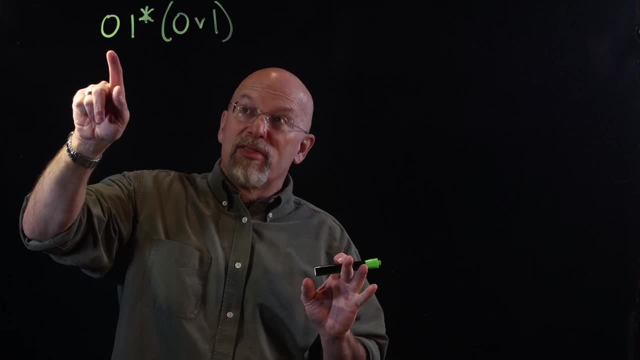 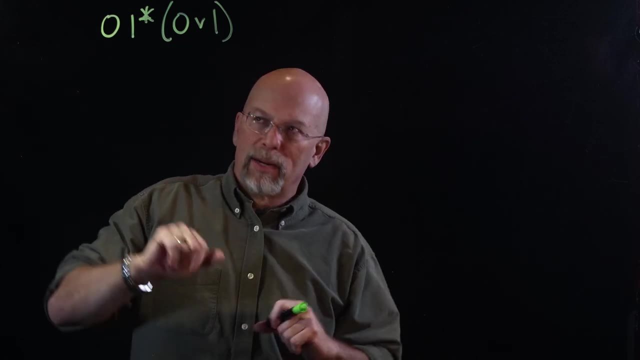 So all the sequences had to start with a 0. Then we may have no 1s, followed by a 0 or a 1.. So 0, 0 was an element, 0, 1 was an element, And then between that first digit and that last, 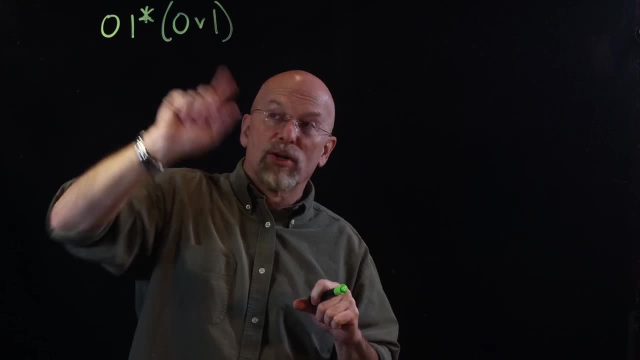 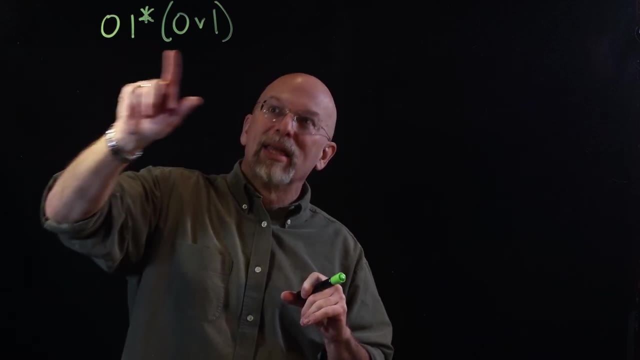 digit, we could have any number of 1s. So we could have 0, 1, 0, 0, 1, 1, 0, 0,, 20, 1s and a 0. Or we could have 0, 1 followed by a 1.. So, as long as we started with a 0, 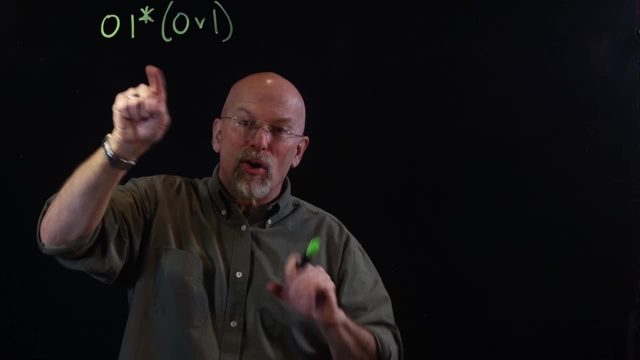 in the first digit we could have any number of 1s. So we could have 0, 1, 0, 0, 1, 1, 0, 0, ended with a 0 or a 1 and had some number of concatenated 1s in between it. we had an. 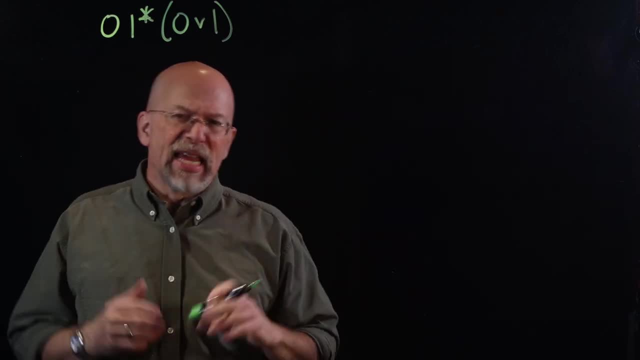 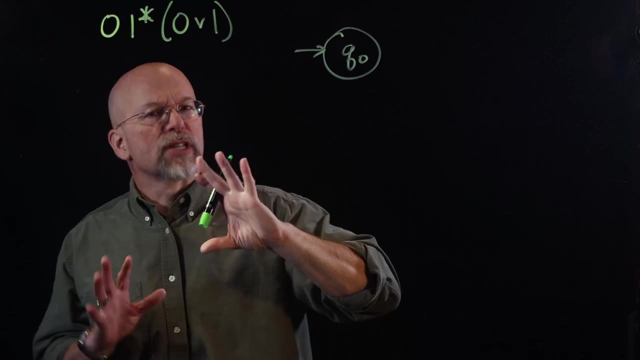 element of that regular set. So what does our finite state automata look like? Well, we're going to do the diagram first. I'm going to start out Q0. That's our initial state. So before we get any bits, before we get any bits from a string, we're going to start out in Q0. 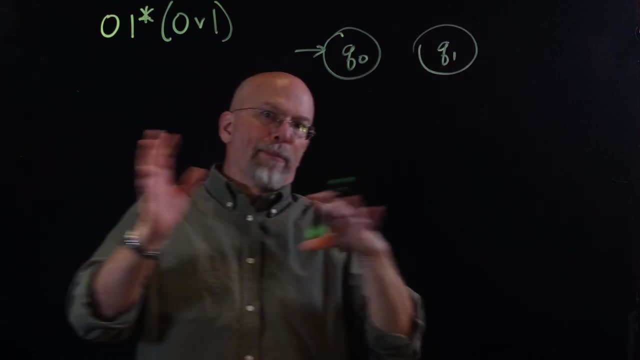 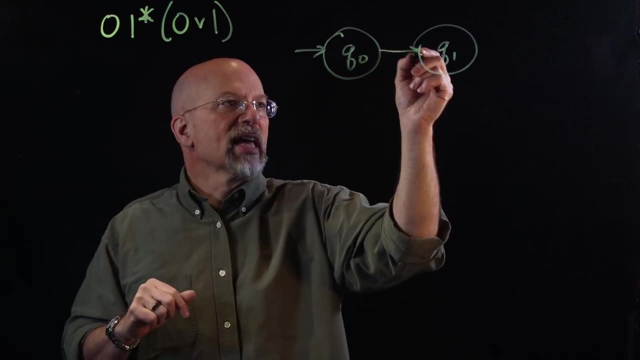 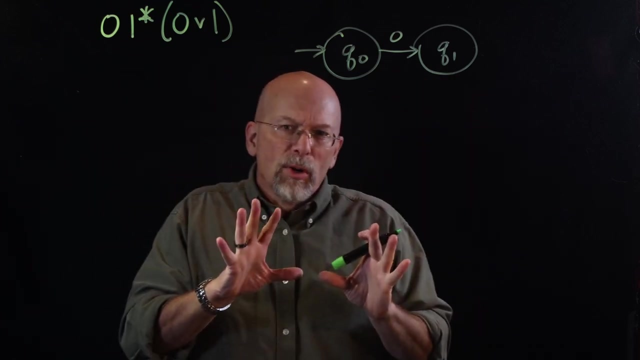 Now the very first element that we're looking for. on our path to finding an element that is a member or a string that's a member of our regular set, the very first thing we have to do is get a 0. That 0 is going to bring us to Q1.. After we've got that 0, then what we're looking. 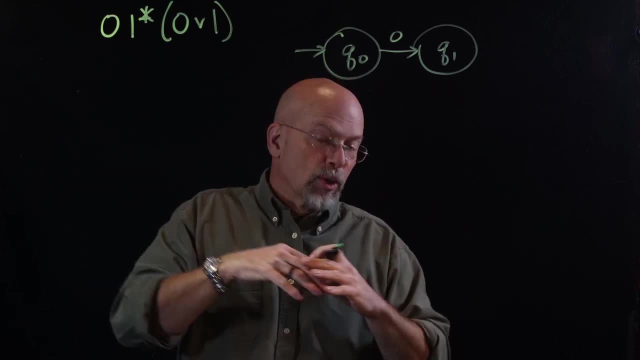 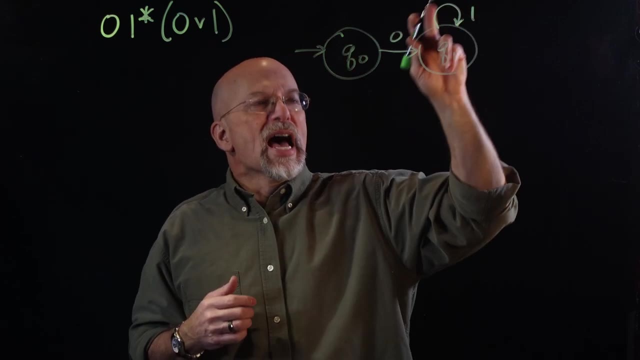 for is any number of 1s. So it could be 0 1s or it could be 1,000 1s, But that's going to give us this little loop here that says: OK, as long as we keep getting 1s, we're going to stay in this. 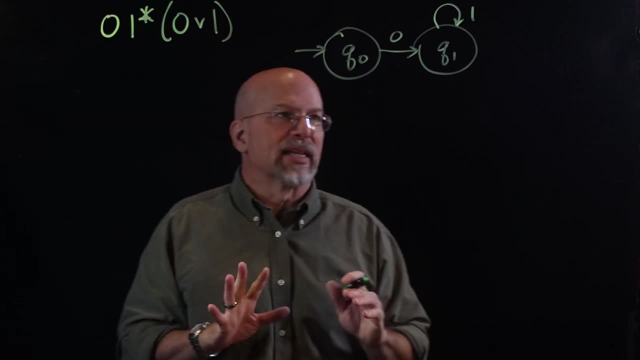 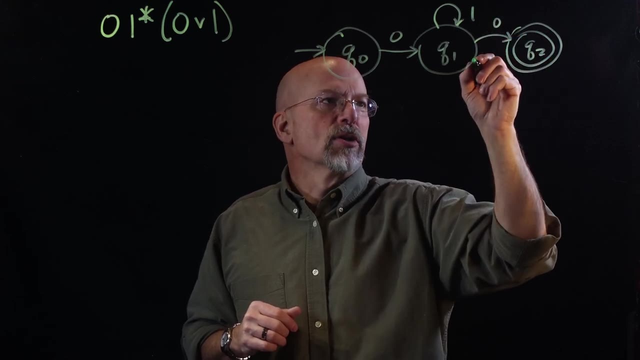 state that says, OK, we're waiting for the final bit. We're going to stay in this state that says OK, we're waiting for the final bit, And that final bit is going to take us to our final state Q2.. And that final bit is going to be either a 0 or a 1.. And so this is our complete state diagram. 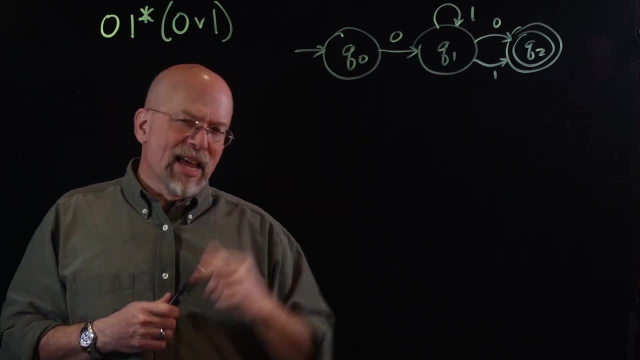 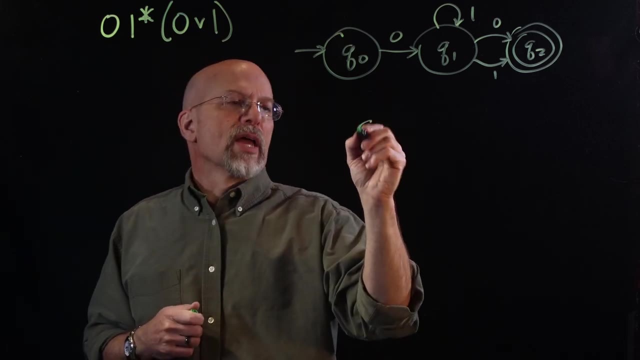 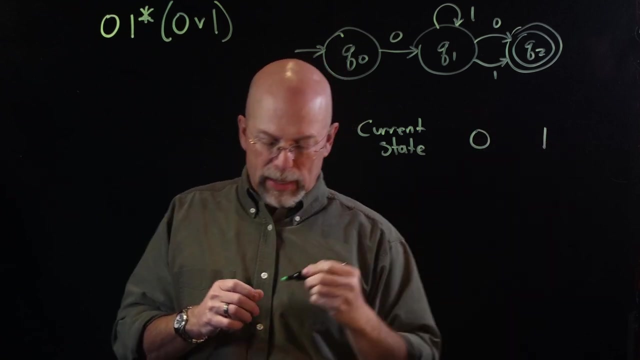 to detect that regular expression. But that's not the only way that we can represent this state machine. Remember, we can represent the state machine with our state transition table. So we have the current state, Then we have what happens if we get a 0?, What happens if we get a 1? And 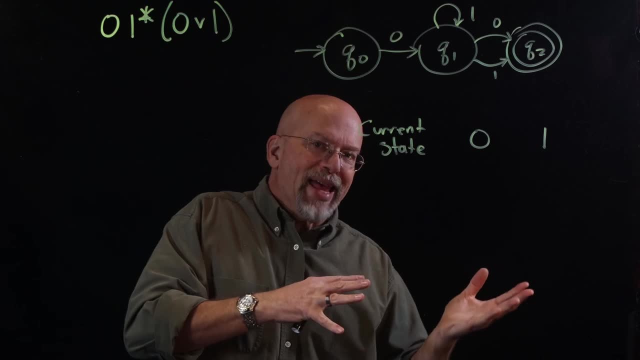 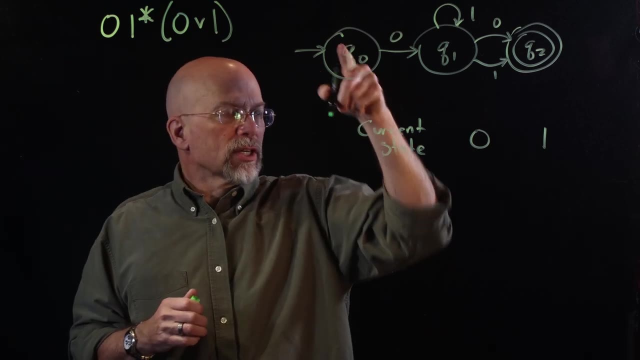 whenever I say what happens, what I mean is: where are we headed? What is the destination From the current state? what's the next state? Well, our first state. we're going to just take a look at Q0. And in fact, let's just go ahead and list all three of these. So we've got Q1. 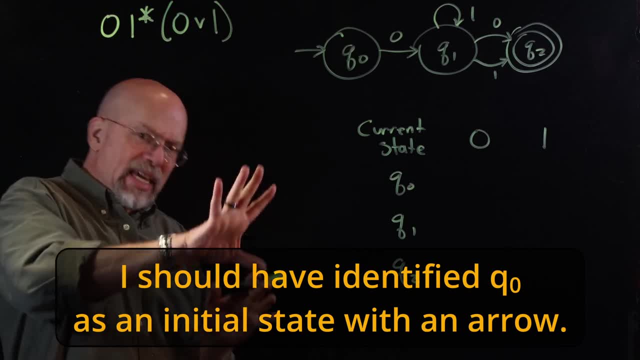 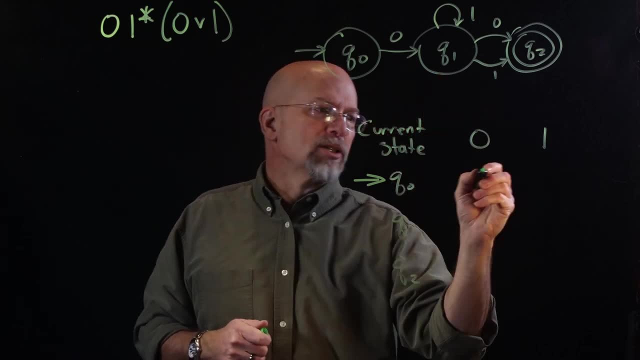 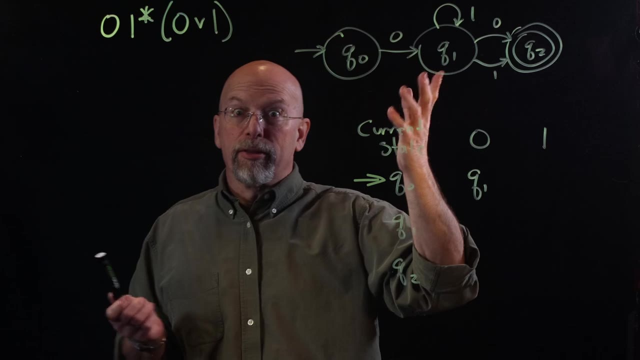 and Q2.. Now these guys, each one of those has a destination based on a 0 or a 1.. Now, if we get a 0 while we're in Q0,, we are headed to state Q1.. If we get a 0 while we're in state Q0, and we get a 1, there's no transition, Nothing is defined. 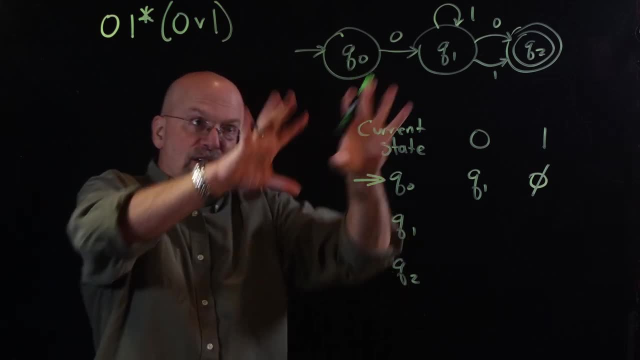 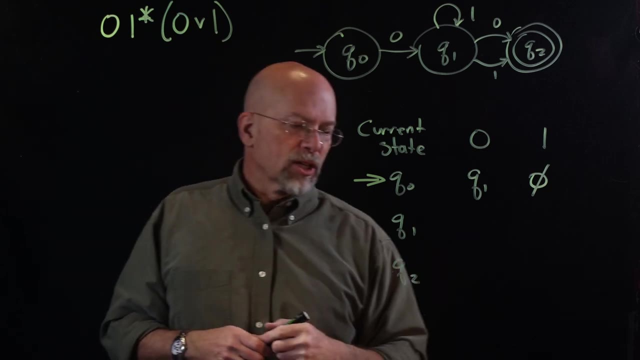 here. This is one of the elements that makes it so that our state machine is non-deterministic yet, And so we put the empty set there, Don't have a destination. Let's take a look at Q1.. When we're in Q1, when we get a 0, very definite, There's one transition that identifies the fact that we 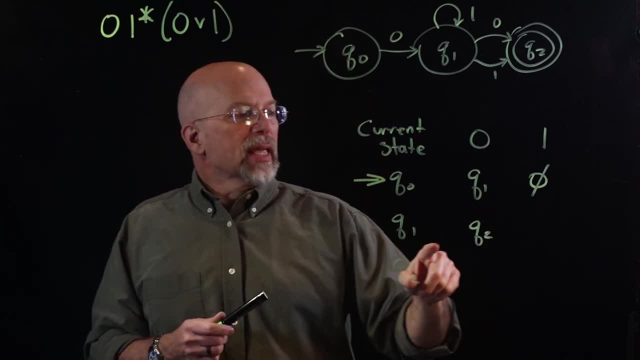 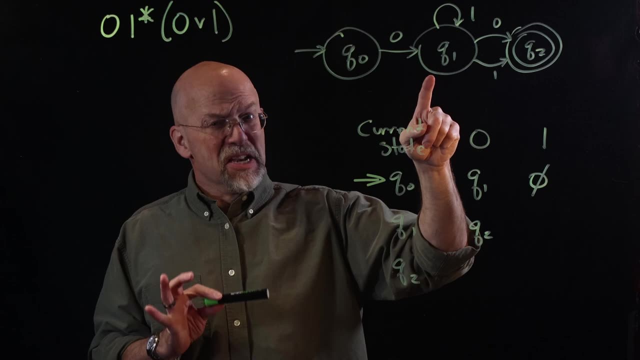 are going to Q2.. If we get a 1 while we are in state Q1,, we are headed to state Q2.. And so we're going to Q1.. If we get a 1, not as exact, not as definite, So we could be coming back to Q1 in the 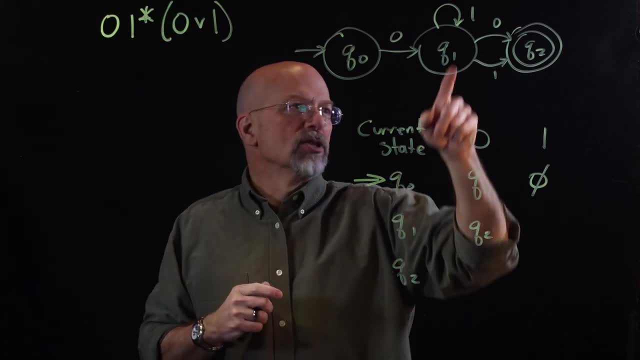 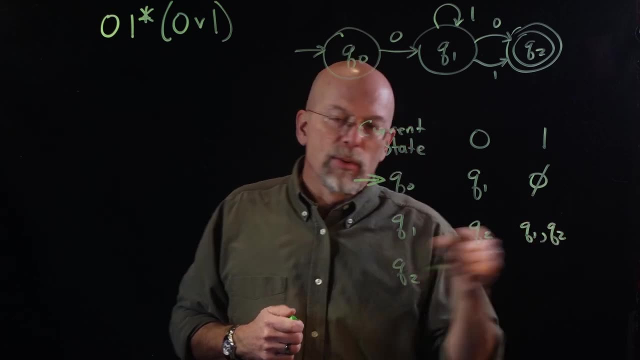 case of getting more elements from the string of 1s, or we could be going to Q2.. So what we actually have here is a set. All right, We could be going to Q1 or Q2.. Now, in Q2, which is our final state, 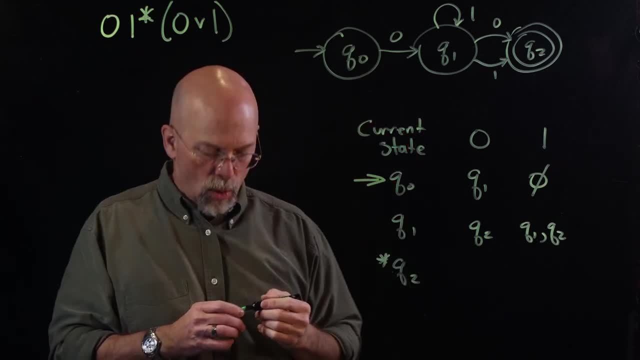 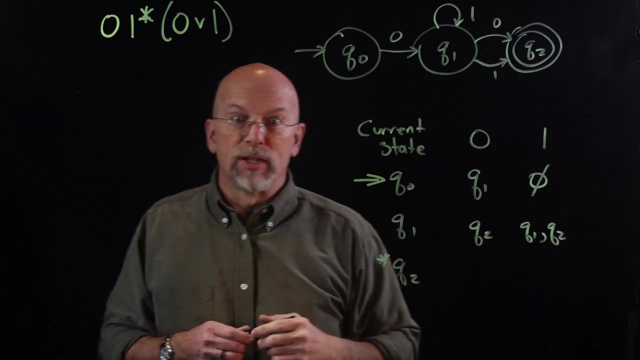 and in our state transition table we're going to identify with an asterisk. If we are in Q2, what happens if we get a 0?? What happens if we get a 1?? Well, there are no transitions out of it. So, once again, we are going to define that or show that state using 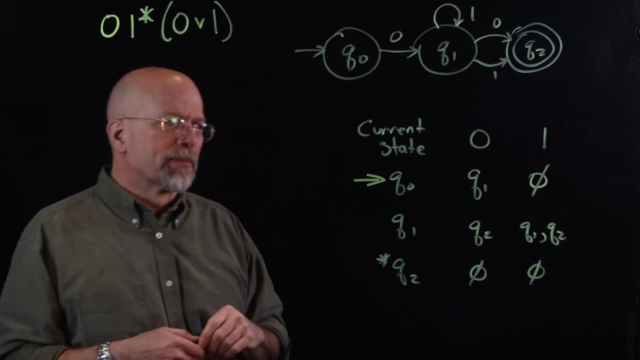 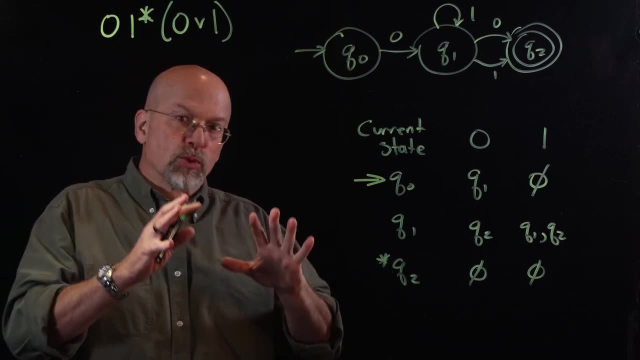 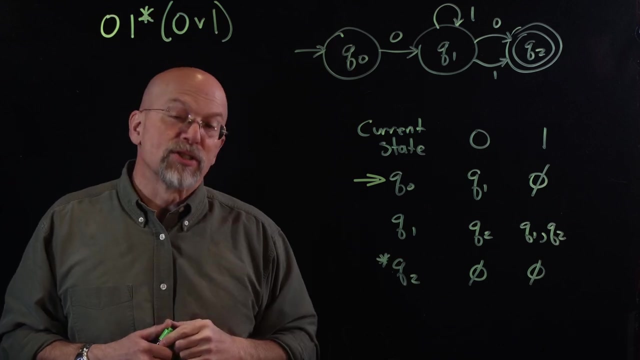 the empty set. Well, that was non-deterministic. Let's take the steps to see if we can convert that non-deterministic one to a deterministic, finite automata. What we're going to do is we're going to leave this state diagram up here and create a new state transition table that represents the 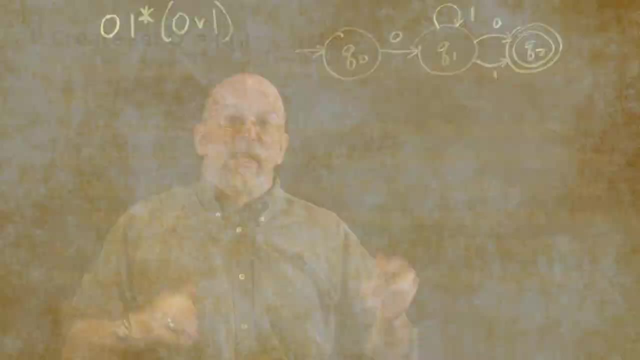 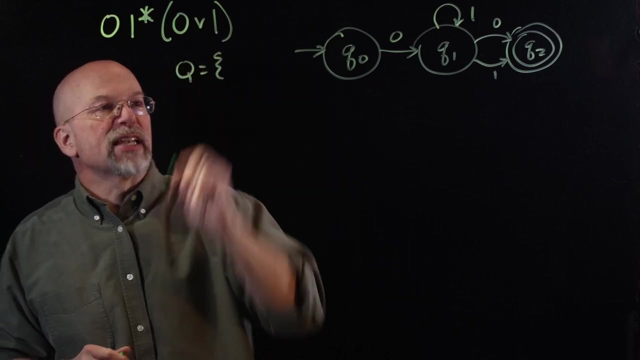 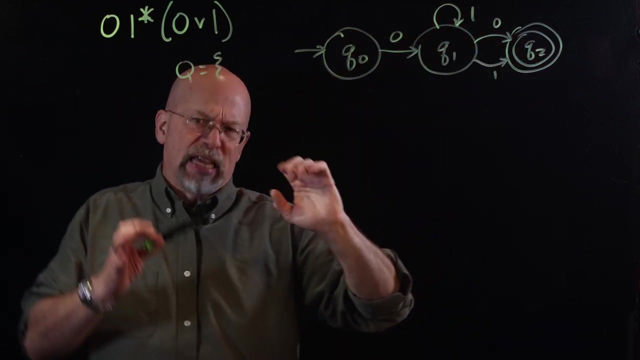 non-deterministic one. Now, remember, our state machines are defined by a number of things. One of the things it's defined by is this set Q, And the set Q is the set of all of the states. So in the case of our non-deterministic state machine we've got: Q is equal to Q0,, Q1,, Q2.. That's all. 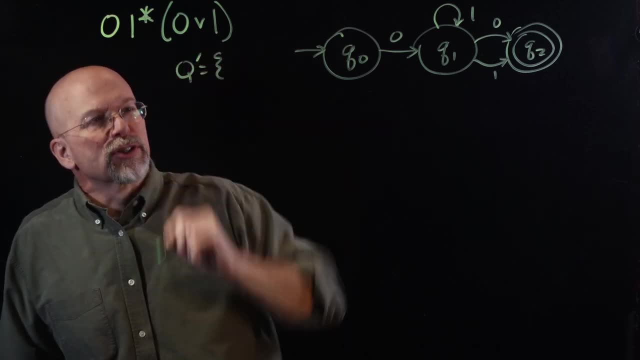 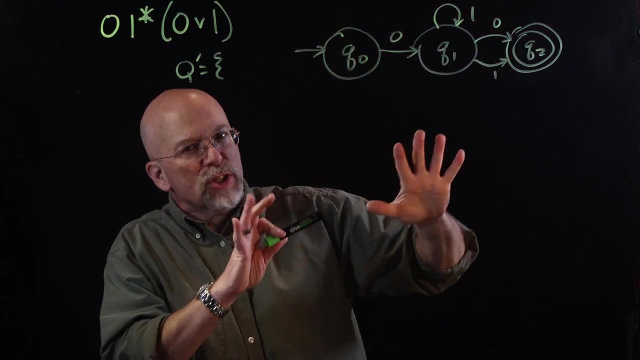 of the states, right. In the case of our deterministic one, the one that we're converting to, I'm going to create a new set of states, So it's going to be based on the set of states we generated for the non-deterministic one, but it's going to have a slightly different organization. 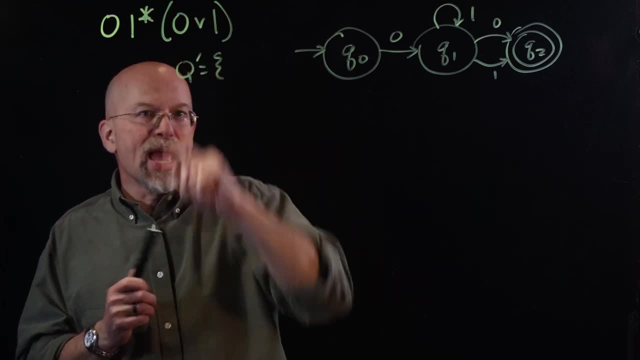 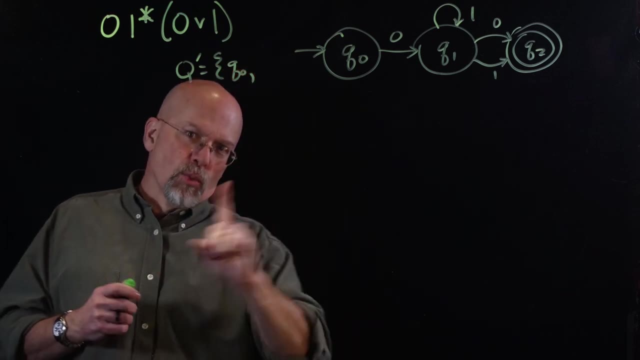 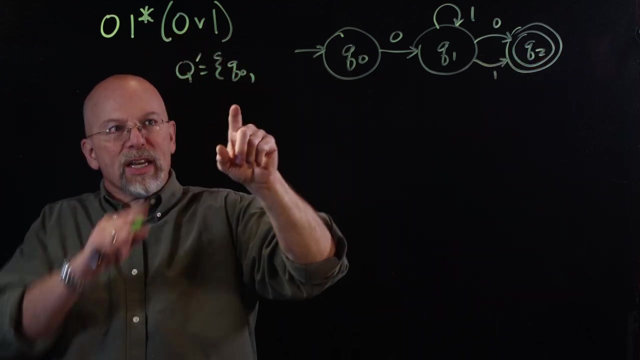 or grouping of these states. Now, the very first state that we add to Q prime is always Q0. We always put Q0, our initial state, And since there's only one initial state, there can be multiple of these accepting states, but there's always one initial state. We put that one initial state. 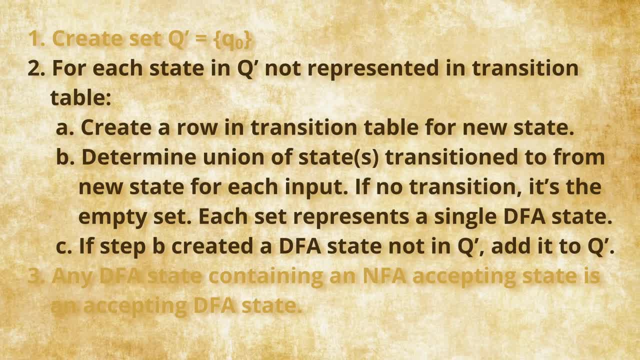 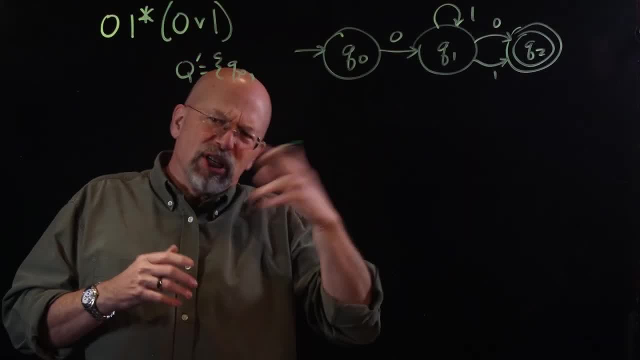 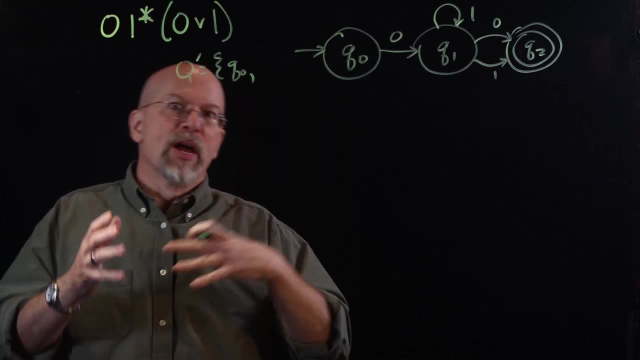 that's the first member of Q prime. Well, that first step was deceptively easy. This next set of steps is actually a loop. It's this iteration based on. any time we create a state that is added to Q prime, we have to add its row in the 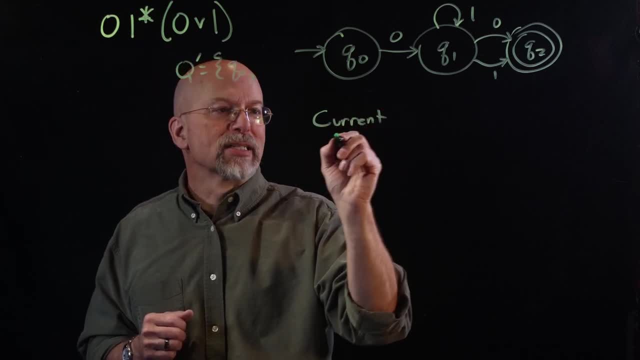 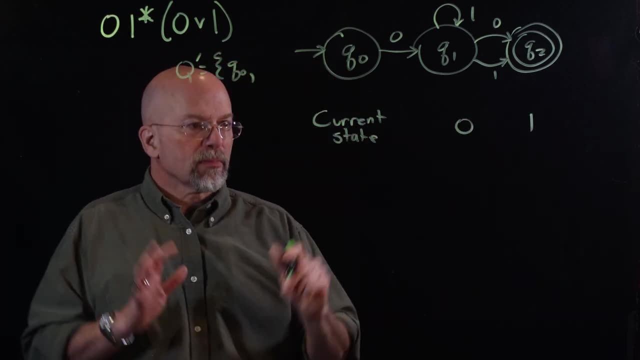 next state transition table. So I'm going to make my next state transition table. There's my current state. There's what happens with a zero. There's what happens with a one. We're going to go ahead and put our initial state in the next state transition table And then we're going to put our 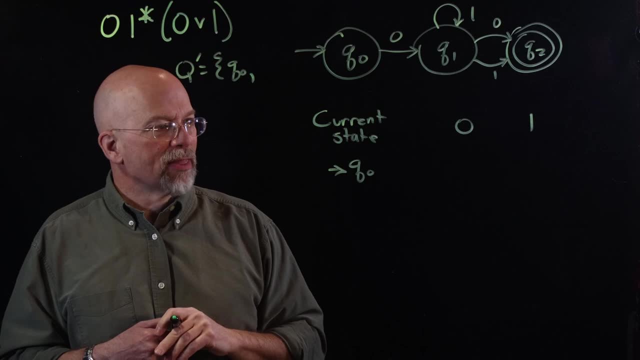 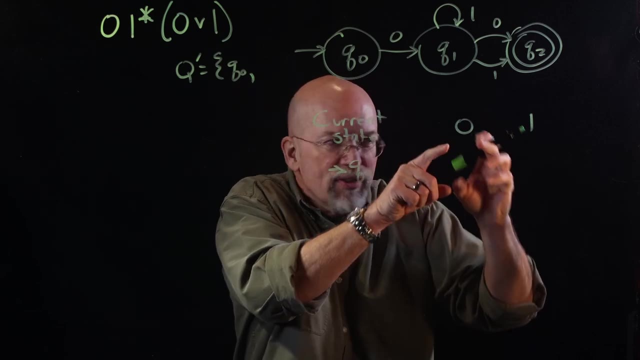 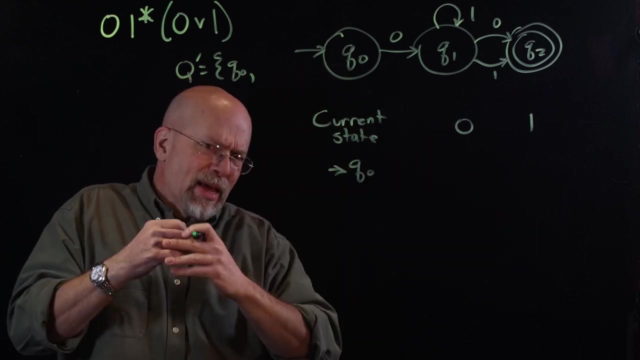 state Q0, put a little arrow there to identify that as our initial state. Now what's going to happen is, as we generate states, each one of these columns is going to get a set of states. It may be the empty set, It may have one destination state, It may have five destination states, but we're 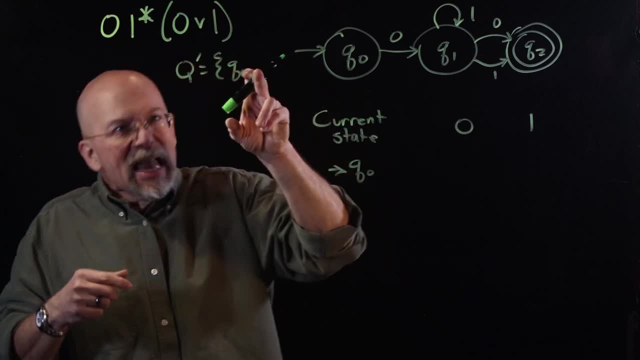 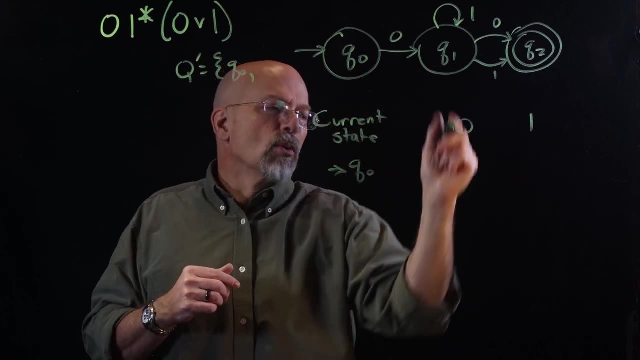 going to group that together as a set And that set is going to become an element of Q prime. Now, when we get a zero, we go to Q1.. All right, So Q1, that's a new state. We're adding it to Q. 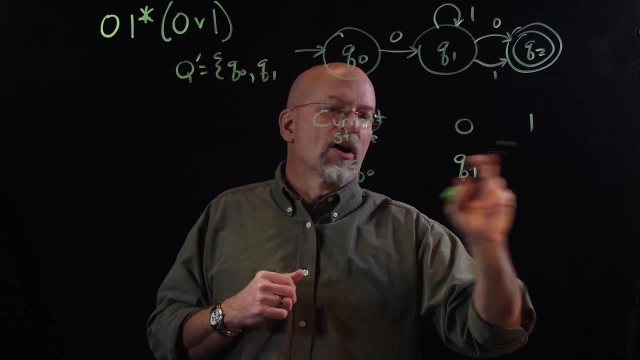 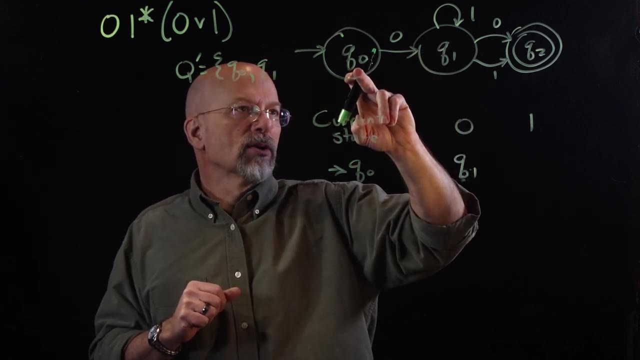 prime If we are in Q0 and we get a one. well, remember from our previous state diagram, we, if we were in Q0 and got a one, we don't know where we're going, So that's actually going to. 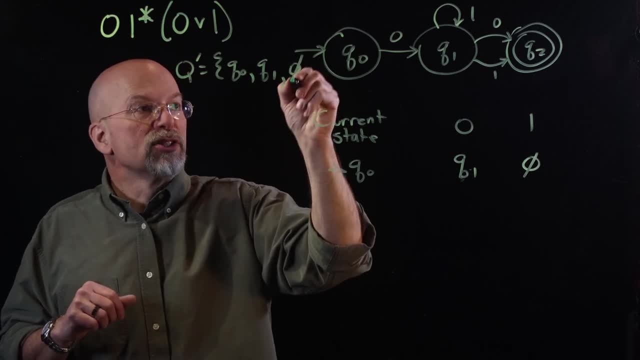 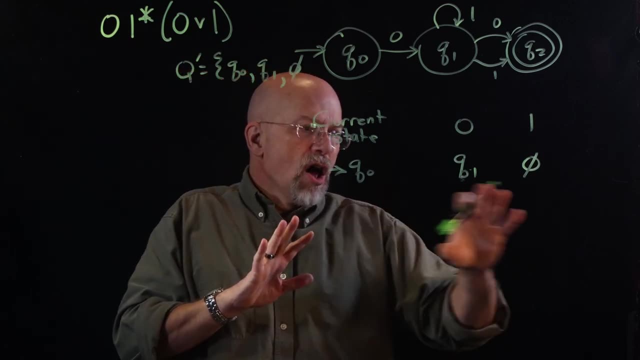 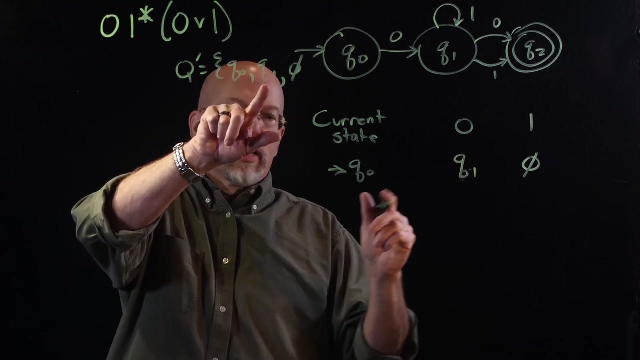 be the empty set. Now it turns out that the empty set is also going to be an element of Q prime. So we now have three states And in fact, all of these are going to become elements in our table. Let's see what the next state is. So we come over here. We've got Q1.. We've added Q1 to Q prime. 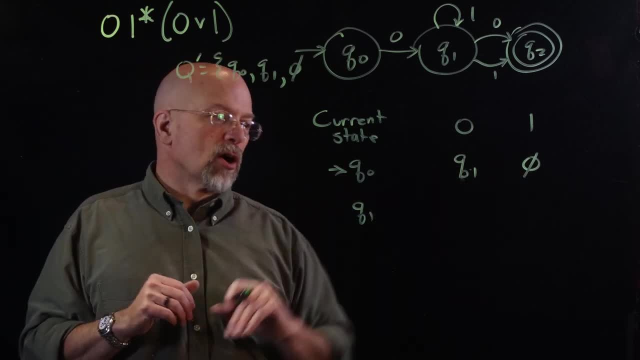 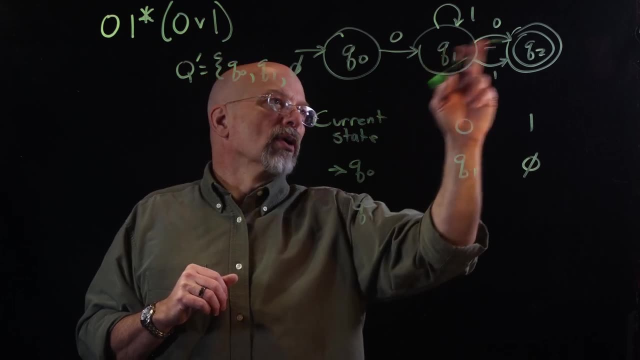 to our set of states, So we need to add a row for it in our transition table. So, Q1, what happens whenever we're in Q1 and we get a zero? Well, if we're in Q1 and we get a zero, 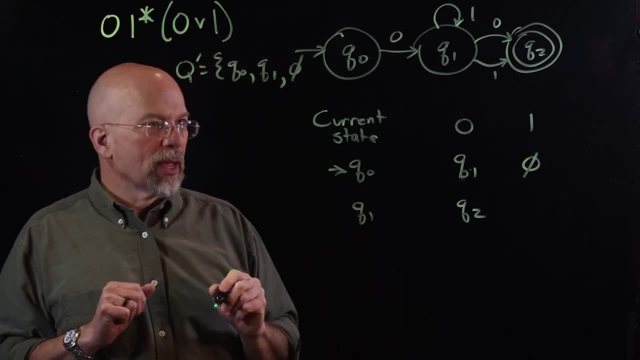 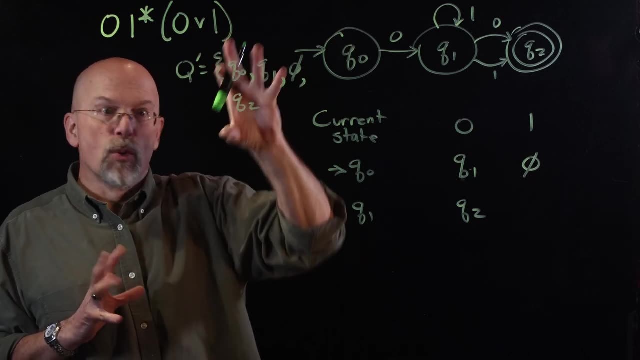 we go to Q2.. Now Q2 is not actually a member yet of our list of states here, So we go ahead and add Q2 to it. So now we actually have four states. We're starting to grow for a few more states than. 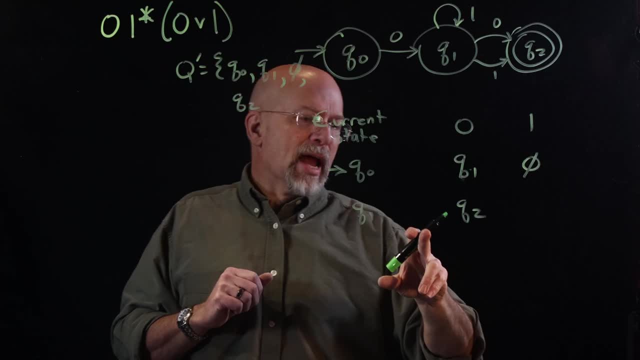 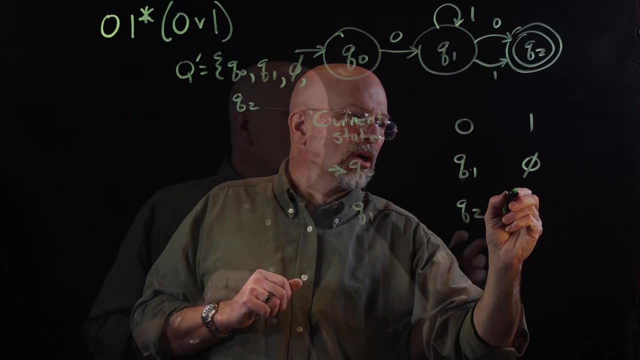 we have in our non-deterministic finite alconada up there. Now, if we are in Q1 and we get a one, we could go to Q1 or we could go to Q2.. So this is actually going to be a set that represents. 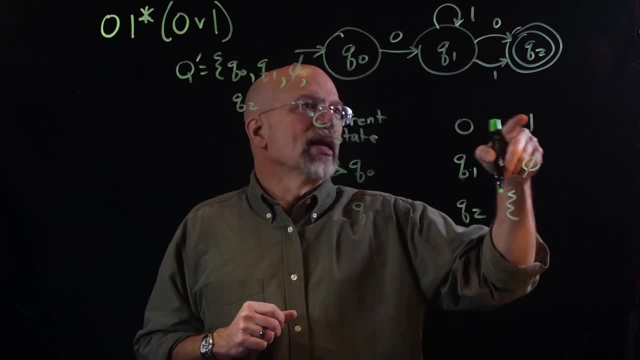 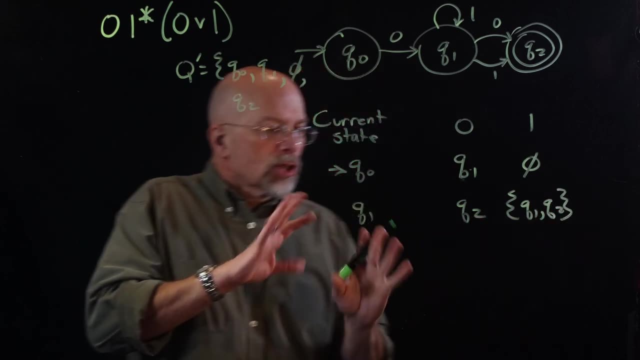 a state. So we go to. if we're in Q1 and we get a zero, we go to Q1 and we get a zero. If we get a one, we go to either Q1 or we go to Q2.. So it turns out that Q1, Q2,. 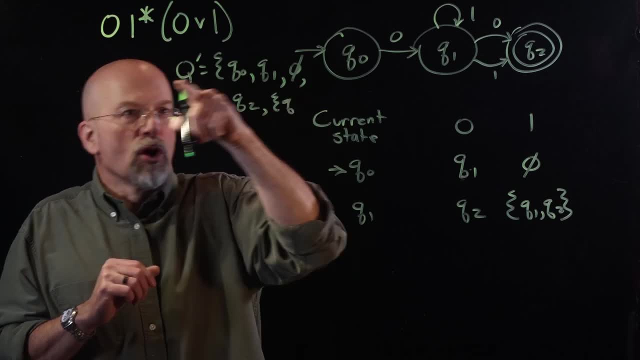 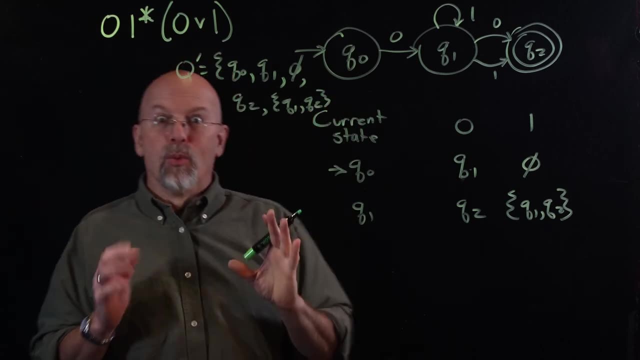 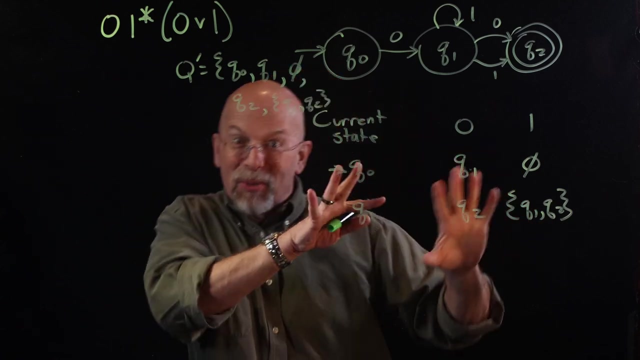 that's actually a state. two for our Q prime here. So we have Q1, Q2, that's actually a state. Wow, We've now got five states for our deterministic finite automata And all of them are represented with just these two rows, or all of them are present as part of our state. So we're. 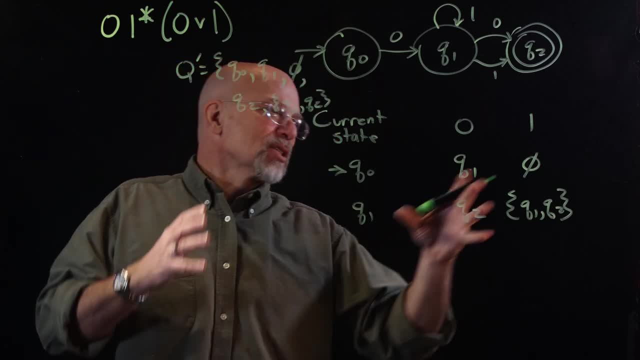 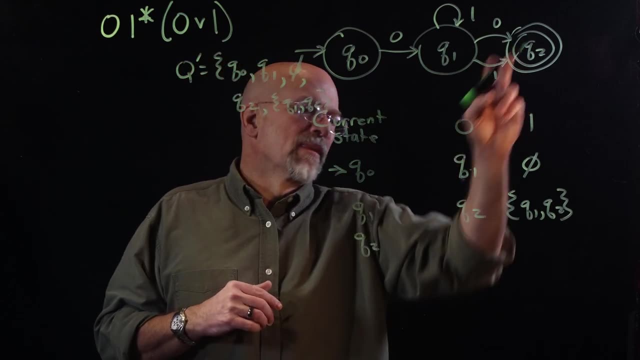 part of these two rows of this next state transition table. Let's pick one of these guys. How about Q2?? Let's say what happens if we're in Q2.. Well, if we're in Q2 and we get a zero? 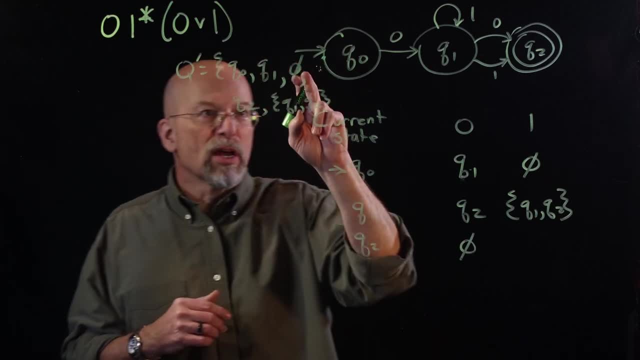 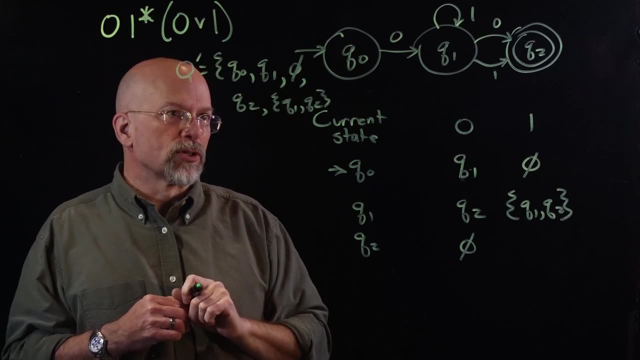 we don't have a transition for that. So that's the empty state. Now we an empty set, So we also have the empty set already in our set of states for the deterministic version of this state, a finite state, automata. So we don't have anything to add If we're in Q2 and we get a one. 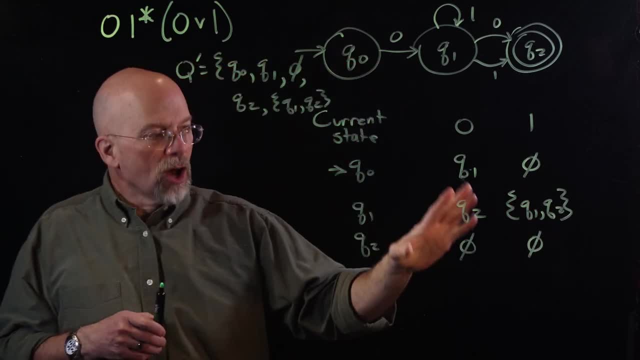 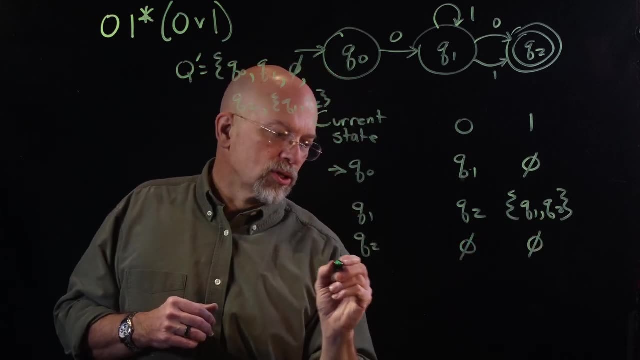 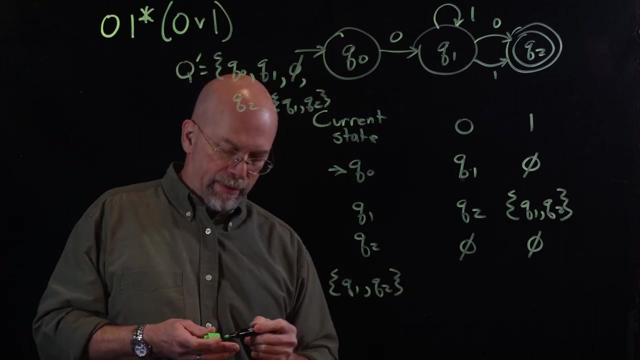 well, we also don't have a destination, So we also have a transition to the empty set. Let's see, Let's pick another one. How about let's do? let's just go ahead and do figure out what happens for Q1 and Q2 whenever we get a zero or a one. This is where things become. 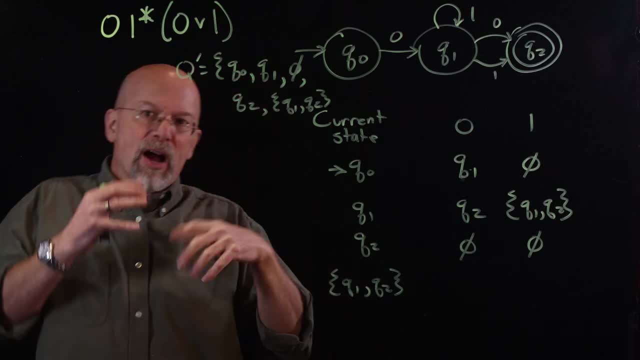 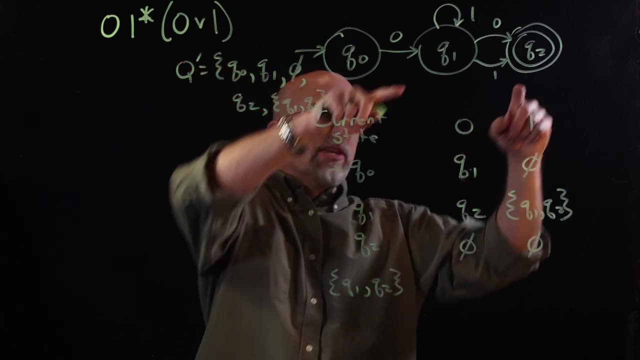 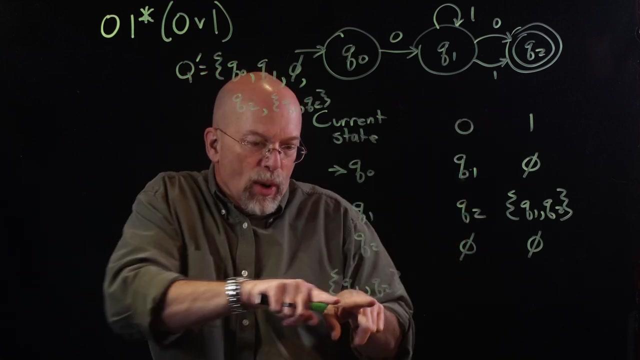 well, not necessarily complicated. You just have to be aware of exactly what our destination is from this newly created state. The newly created state is really the union of Q1 and Q2.. So what you want to do is say: where am I headed when I get a zero, if I'm in Q1 or if I'm in Q2? So it's the union of those two. 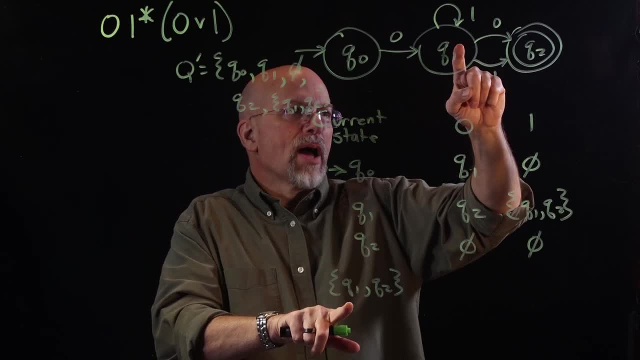 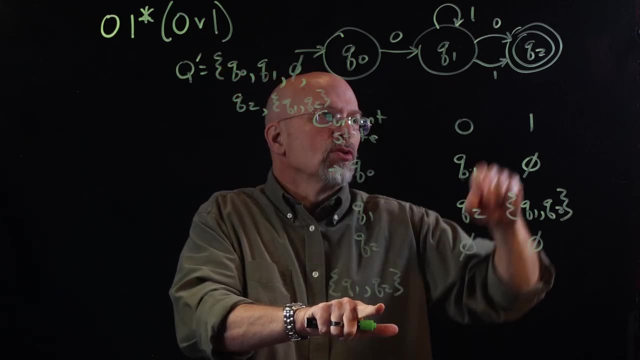 So if I'm in Q1 and I get a zero, I'm headed to Q2.. So Q2 is going to be one of the elements of the set that is going to be our destination here. If I'm in Q2 and I get a zero, I'm headed to. 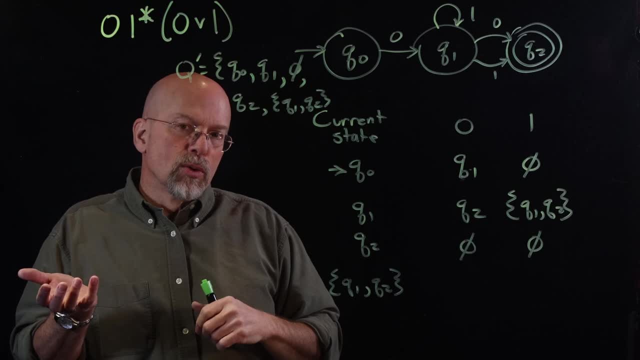 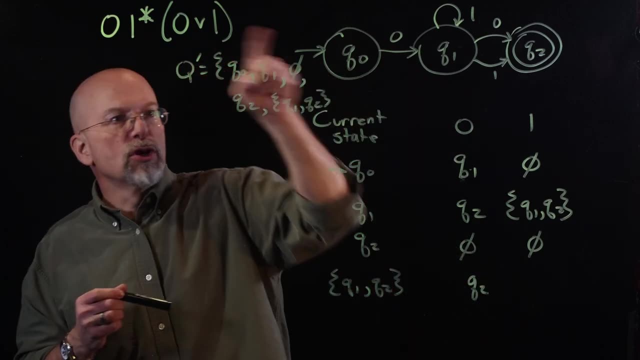 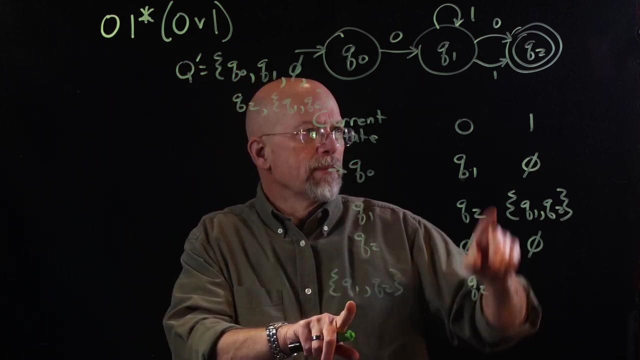 the empty set. So what's the union? The union of Q2 with the empty set Turns out, it's just Q2.. All right, Now we already have Q2 in our set up here. So Q2, we don't need to add. What happens if we're in Q1 or Q2 and we get a one? 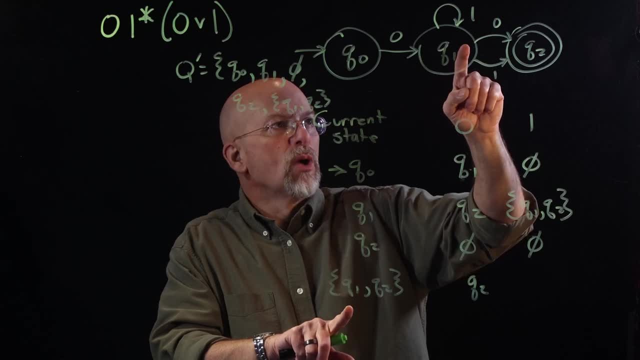 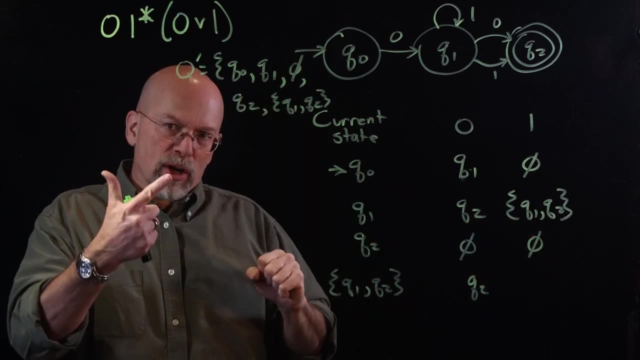 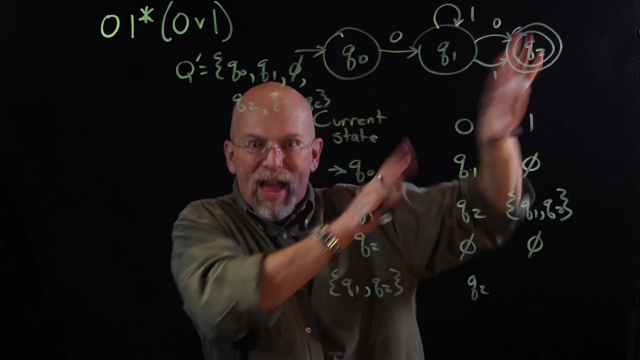 Where are we headed? Well, if I'm in Q1 and I get a one, I'm headed to either Q1 or Q2.. So there's two elements of this destination set: Q1, Q2.. If I'm in Q2 and I get a one, I'm headed to the empty set. right, I don't have. I don't have a. 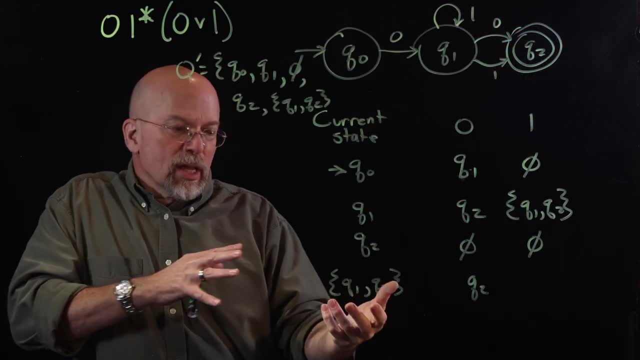 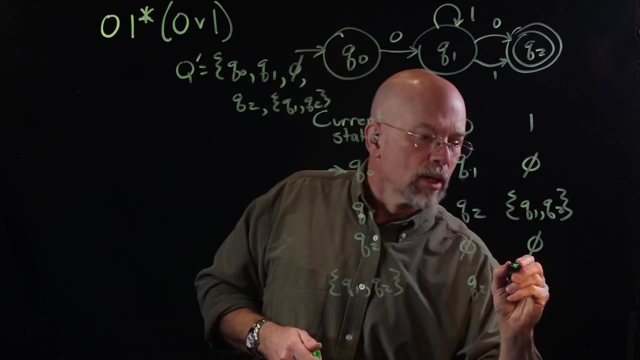 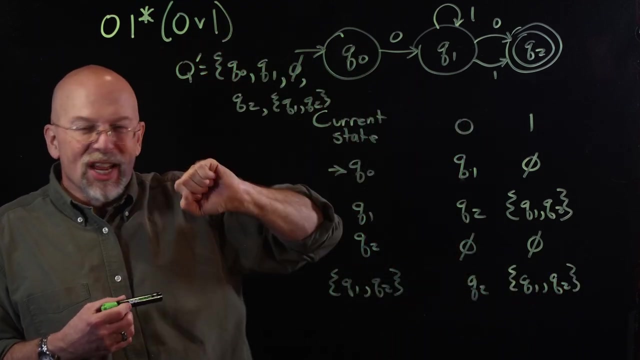 destination there, So Q, the union of all the destinations for Q1 or Q2, whenever I have a one is Q1, Q2.. Already a member of our next of our, of our states for the deterministic finite automata. 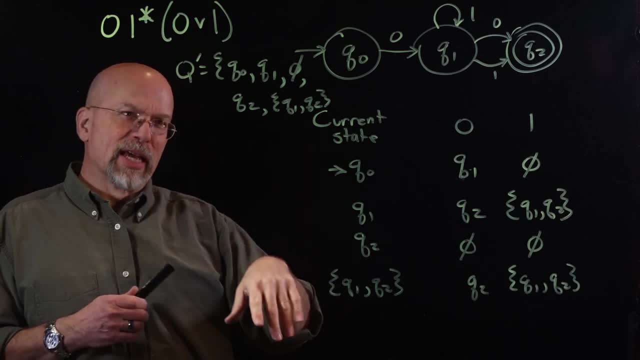 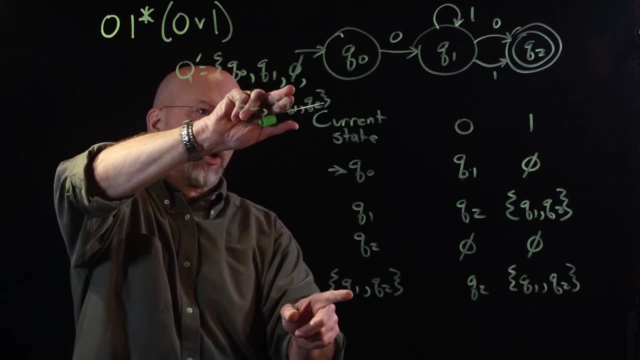 So I don't have anything, Do I have all my states? Well, I've got Q0,, I've got Q1,, I've got Q2,, I've got Q1,, Q2.. What I don't have is the empty set. So I also have to define that, because it is one of the 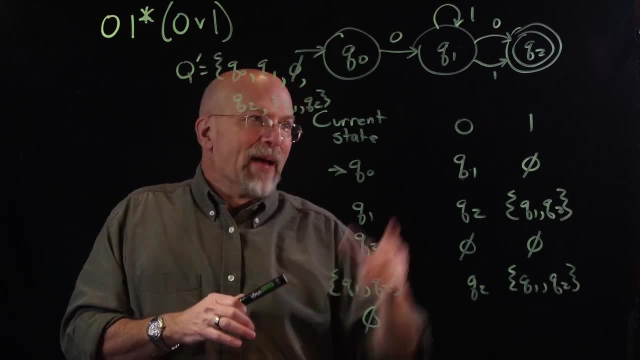 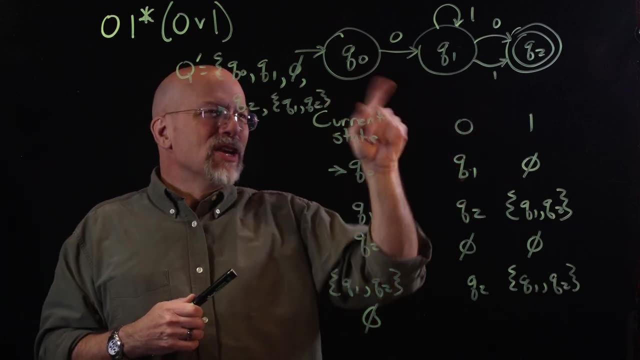 elements of our states. When I have. when I'm in the empty set state. when I'm in the empty set state: yes. whenever I'm nowhere right: No. whenever I'm in the. whenever I'm in no state. 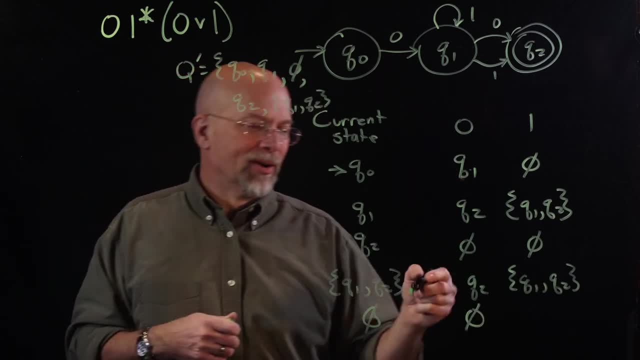 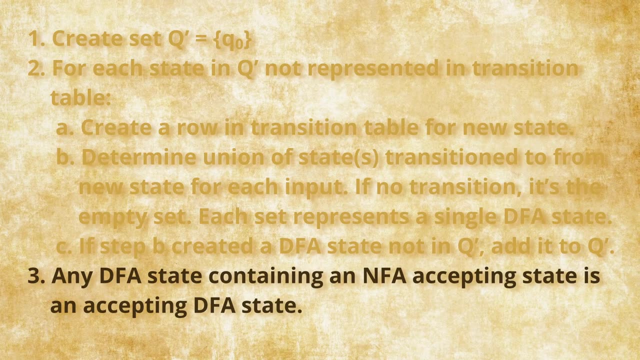 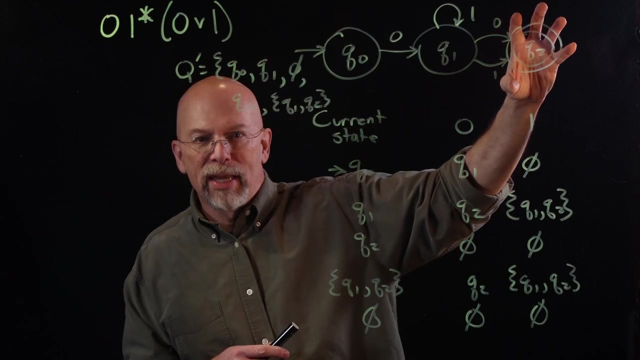 where am I headed? If I get a zero, I'm headed Nowhere. If I'm in nowhere, I'm in the empty set. and I get a one, I'm also headed to nowhere. Now, from our non-deterministic, finite automata, you can see, we have this one accepting state. 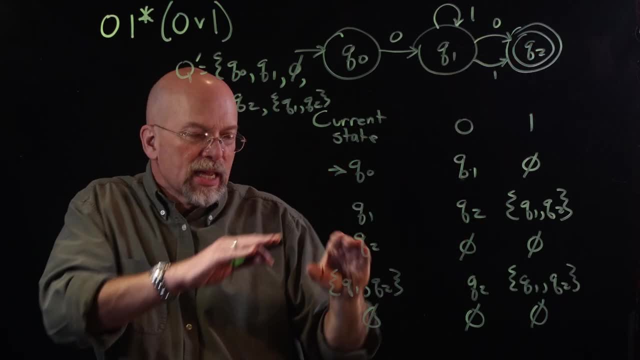 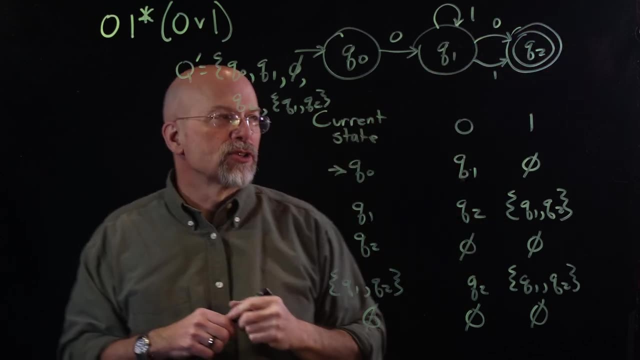 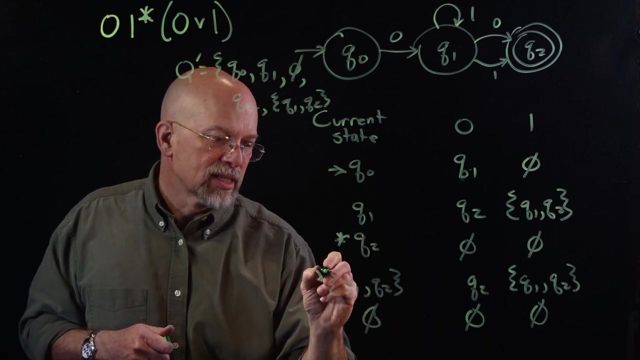 Well, looking through this list of states here, we're going to identify every row that has a state that contains this accepting state from the original non-deterministic one. Well, Q2 is here and Q2 is contained in this set, So those two are both accepting states, None of the other. 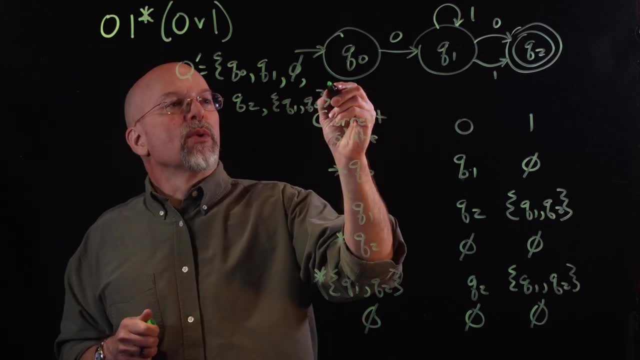 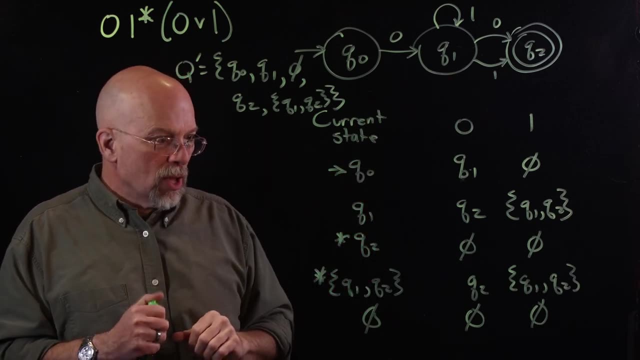 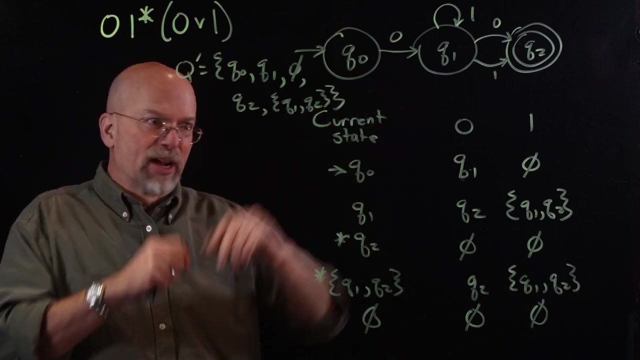 states are accepting states. So we've got all of our states here in Q prime, And the other thing we've got is this state transition table. Well, it defines everything that we need in order to determine what our deterministic finite automata state diagram should look like. We've got the list. 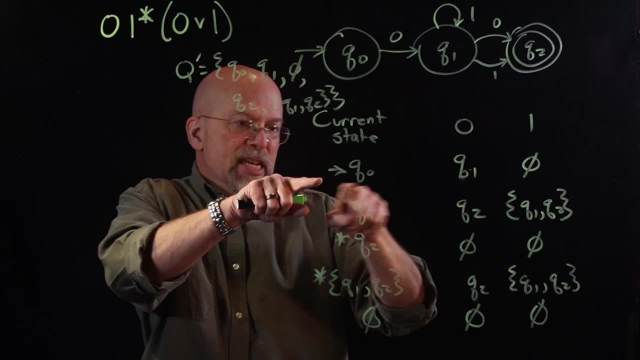 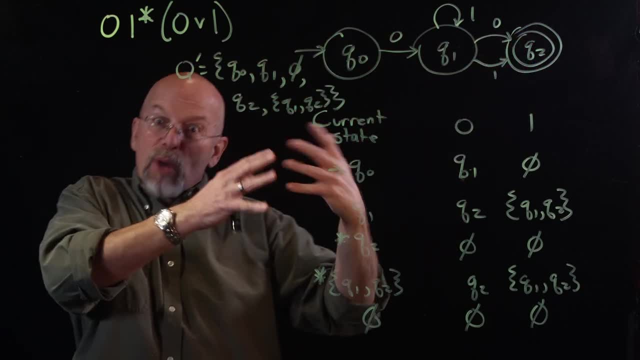 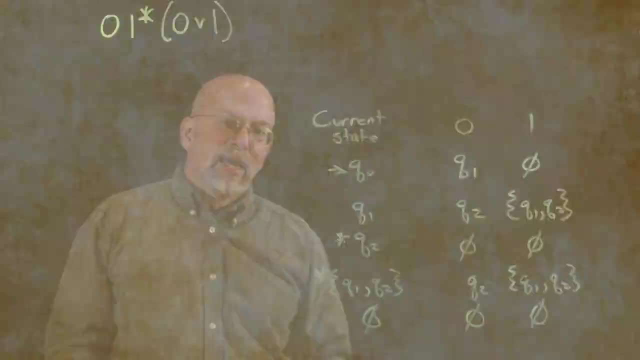 transitions. We can now get rid of this guy because we don't need it as a reference anymore Now. we're going to make our deterministic one Now, in order to make things a little bit clearer or a little bit simpler whenever I'm drawing my 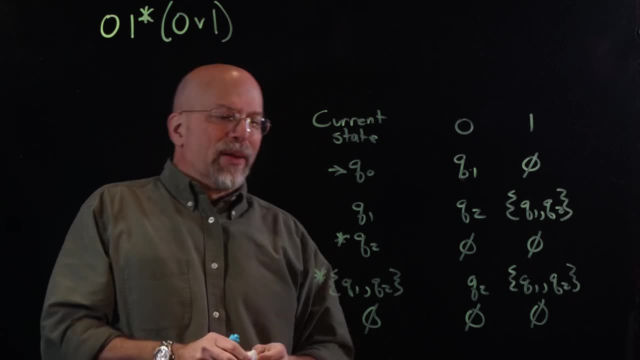 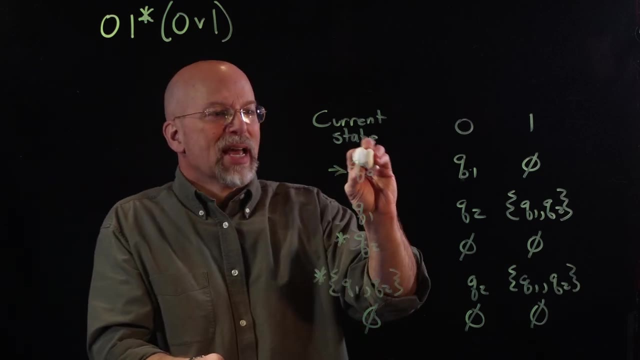 state diagram. I'm going to clean this up by, instead of using sets to represent each one of the states, instead, what I'm going to do is I'm going to use new state names. Now, to keep things simple, I'm going to go with a different set of letters. So Q0,, I am just going to 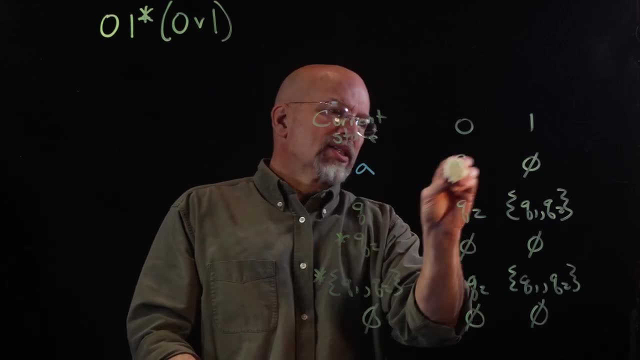 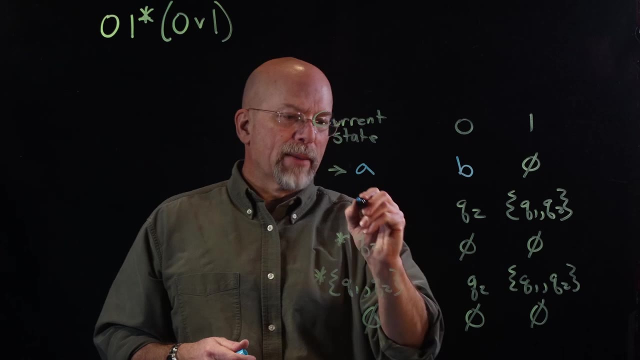 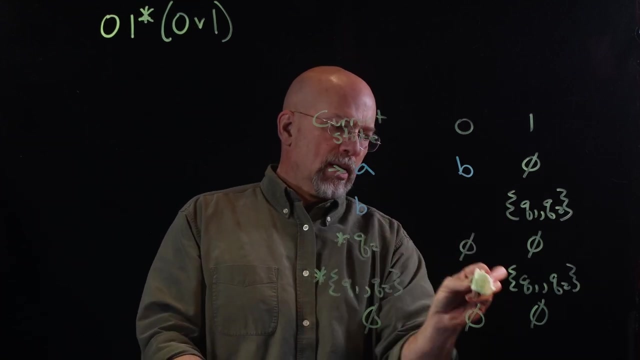 represent with A Q1, let's see, Q1 is there and there. There's no other sets where I see Q1.. So that I'm going to call B. Let's see how about Q2? Q2 is here, here and here That I'm going to. 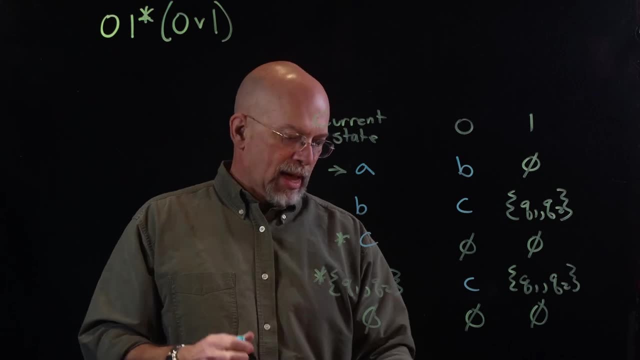 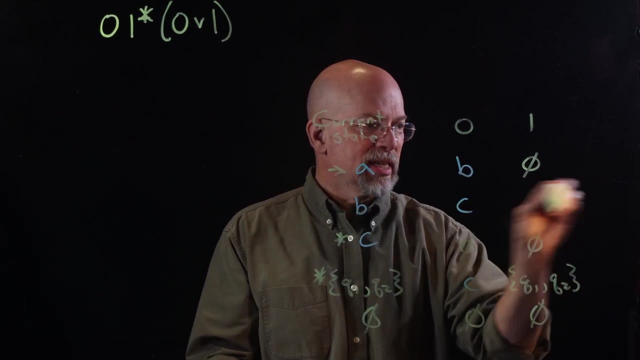 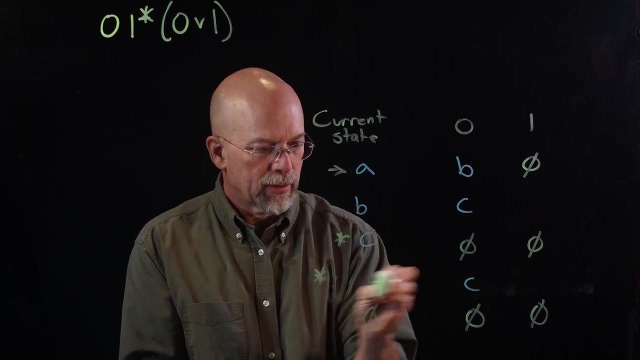 represent with C. Okay, And then this wonderful large set Q1, Q2,- this one I'm going to represent with D. So let's go ahead and clear these three guys up. All right, Not as clean as I'd like it to be, but we've got. 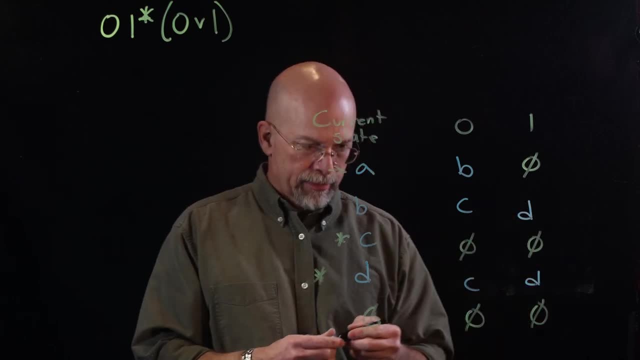 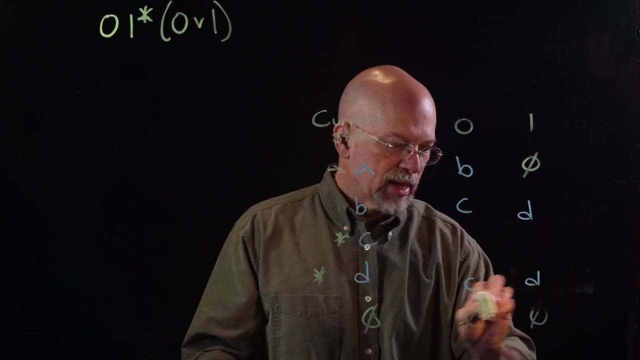 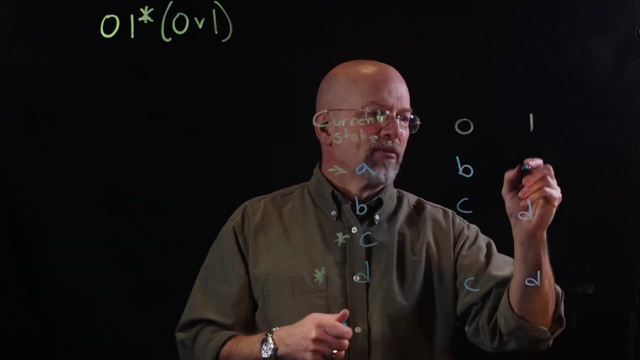 D, D and D, And then the empty set. The empty set appears in a lot of places, So we're going to clear those two lines, Those two elements, those two elements that row and that, And now we have E, E, E, E, E and E. 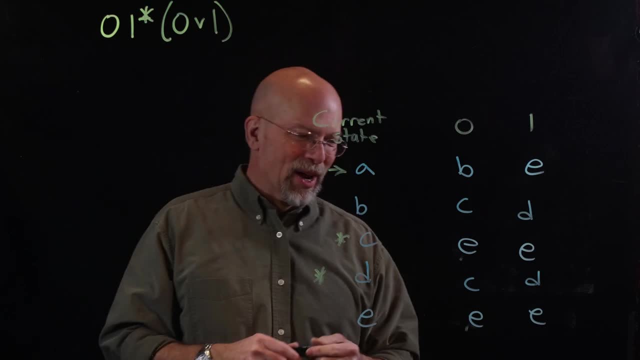 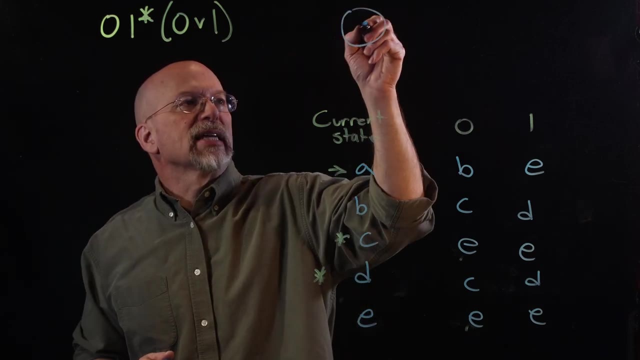 All right, So there's our new state diagram, or, excuse me, my new state transition table. What does the state diagram look like? Our initial state is state A, So we put our arrow in there to indicate that A is our initial state. If we get a zero, we get a zero. So if we get a zero, we get a zero. 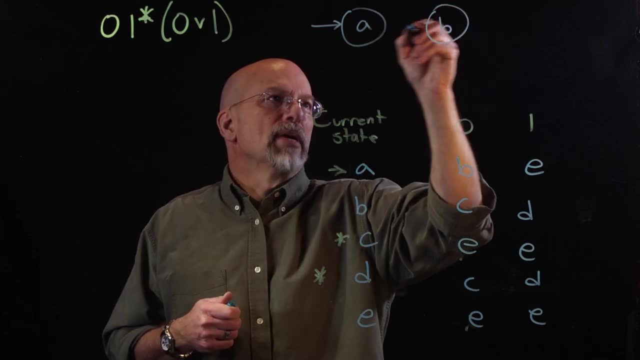 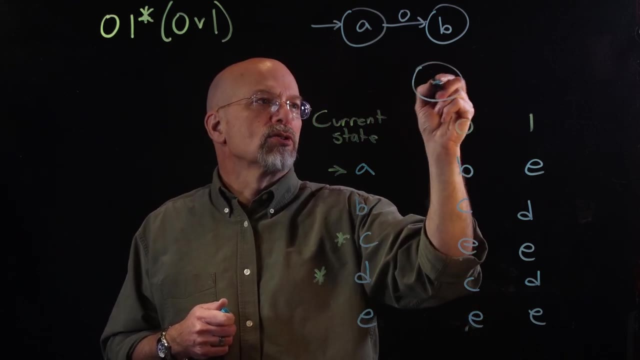 We've got a transition coming out of A that goes to B. So a zero will take us to B, A one, when we're in state A, will take us to state E. Now the key is is that our input alphabet has two. 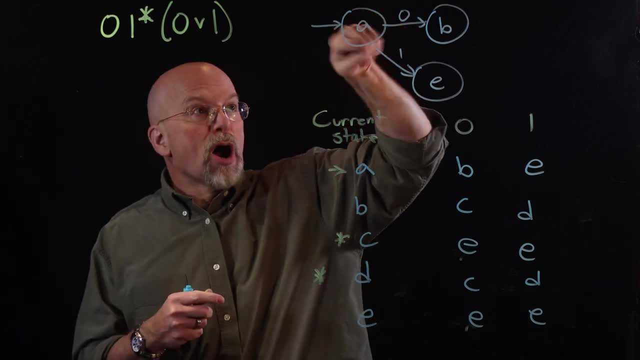 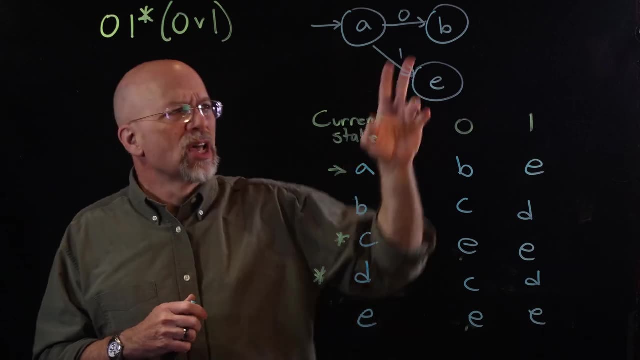 elements. It's the binary alphabet. It's either a zero or a one. So the number of transitions coming out of A need to account for both the zero and the one, and it does. But B and E they still need to have zero and one transition. So we've got a transition coming out of A that goes to B. 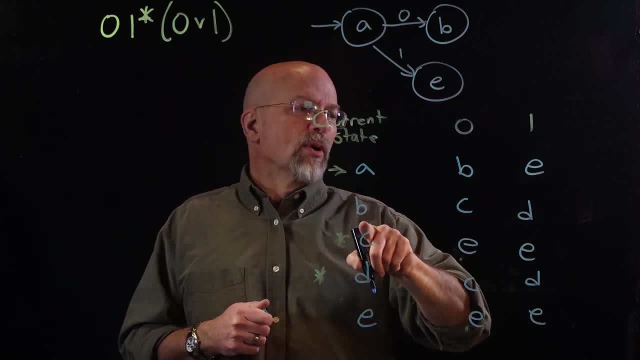 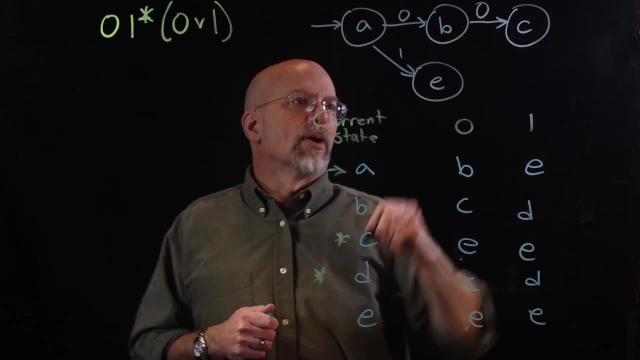 Let's go ahead and do B. So if we're in B and we get a zero, we're going to state C. All right, So that's a zero. If we're in state B and we get a one, we're going to state D. So we've got state D. 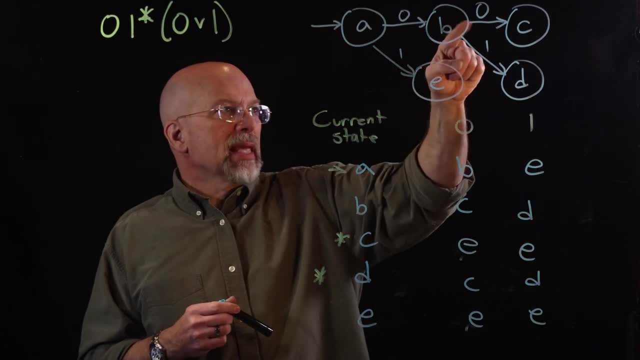 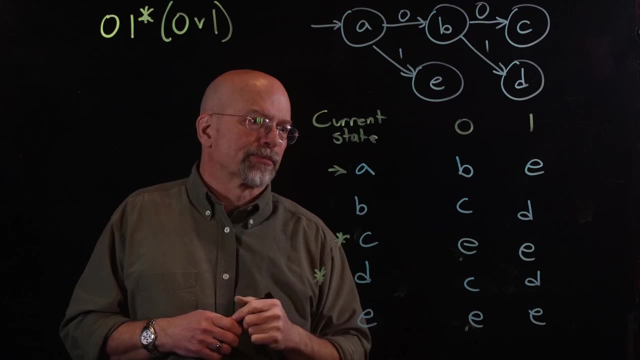 here if we get a one. So now, coming out of B, I have both my zero and my one, But these three states- C, D, E- we don't have our zero and one transitions out of them yet. Now let's take a look. 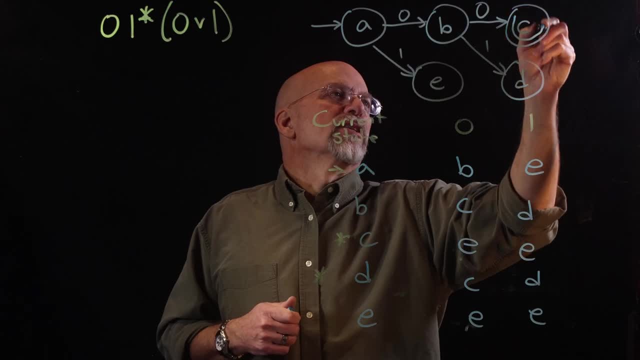 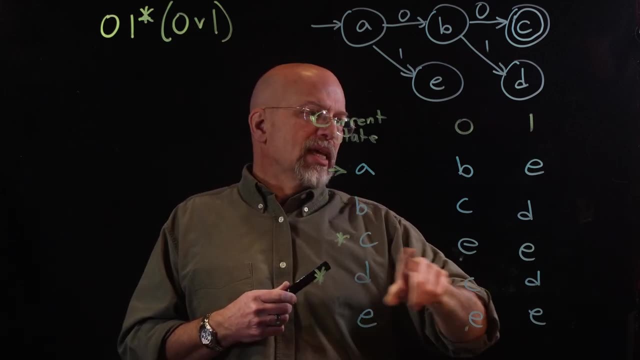 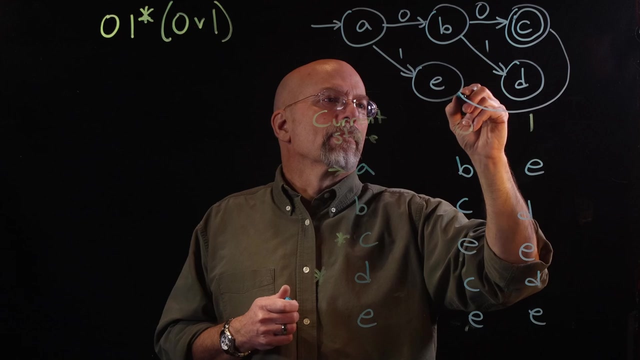 at C. C is an accepting state. So we put a double circle around that one to show in our diagram that it's an accepting state. If we are in C and we get a zero, then we go to E. All right, That's for a. 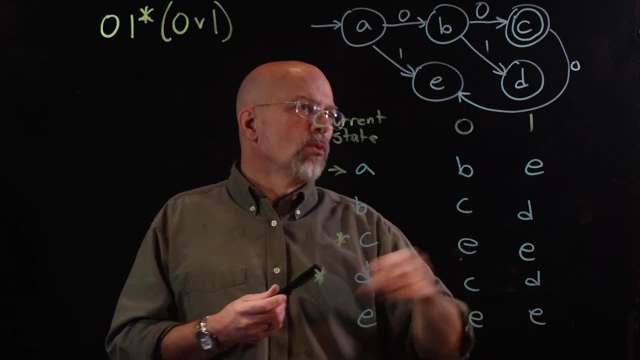 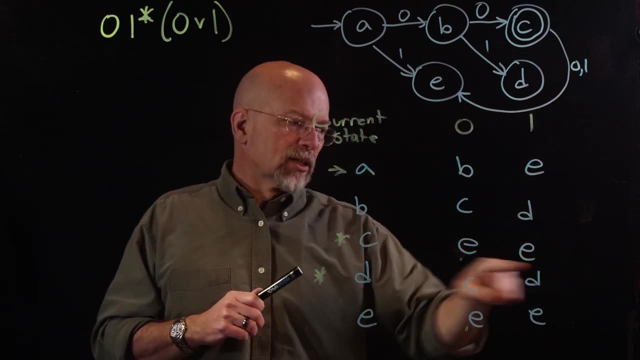 zero. If we're in state C and we get a one, we also go to state E. So from C, we now know what happens if we get a zero or a one. Now let's take a look at D. If I'm in D and I get a zero, then that means I'm headed up to state C. 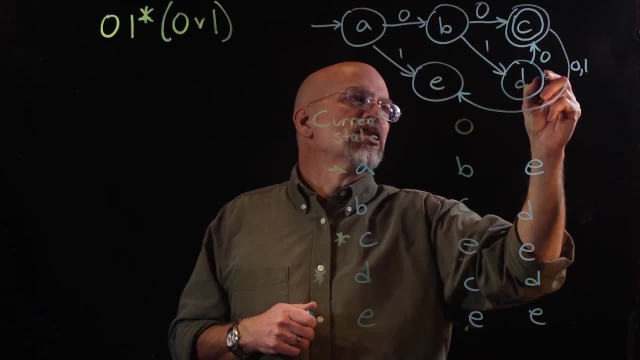 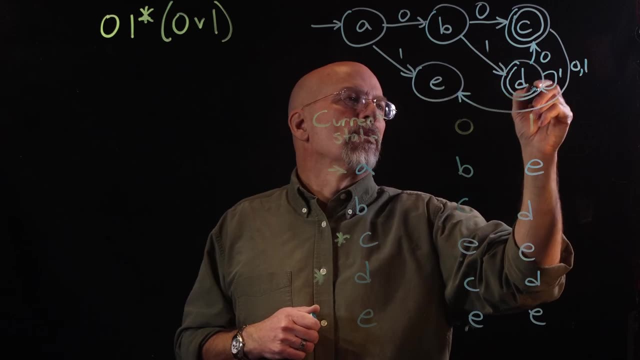 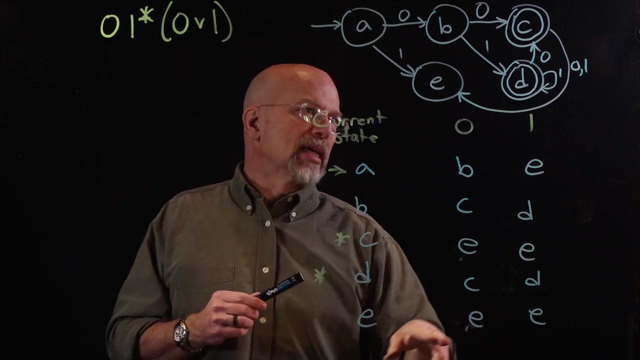 If I'm in D and I get a one, then I stay in state D. Notice also that D is an accepting state, So we put the double circle around that one too. And then, lastly, if I'm in state E, so I've got zero. 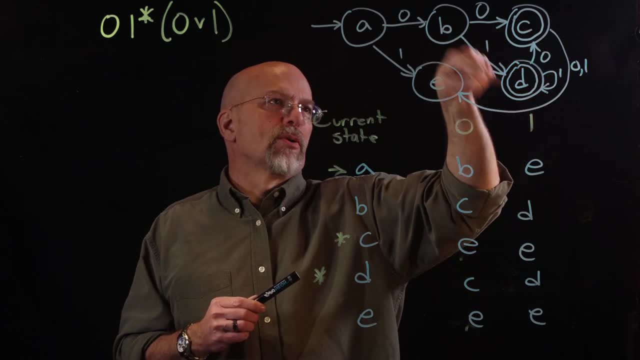 and one coming out of D, I've got zero, and one coming out of C- zero and one coming out of B- zero and one coming out of A. E is the last state If I'm in E and I get a zero. 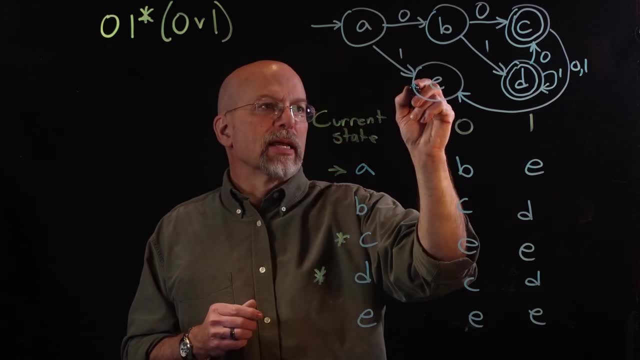 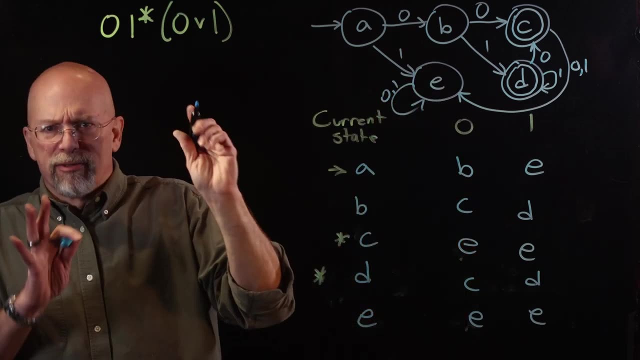 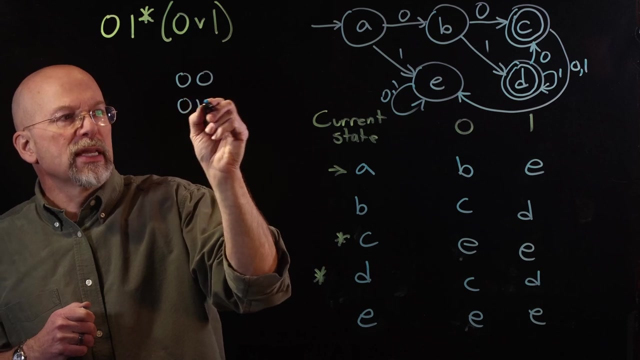 or if I get a one, I'm headed back to state E. Does this make sense? Well, remember, we had a couple of examples for things that adhere to this regular expression If it began and ended with a zero, with any number of ones in between it. 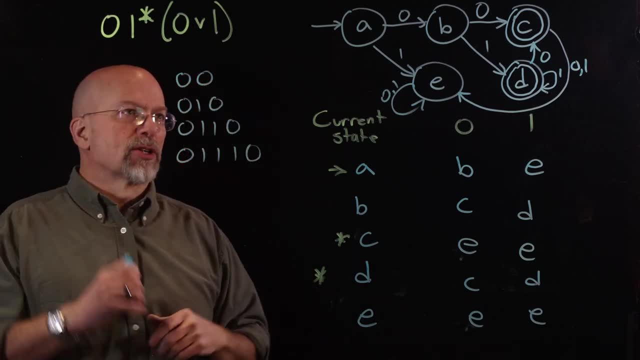 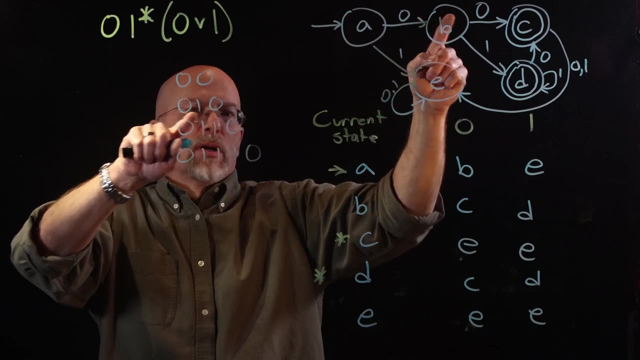 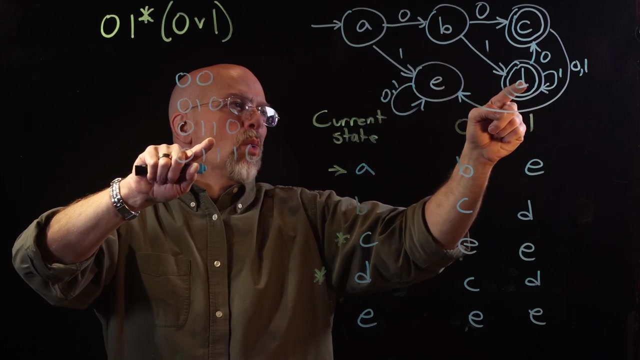 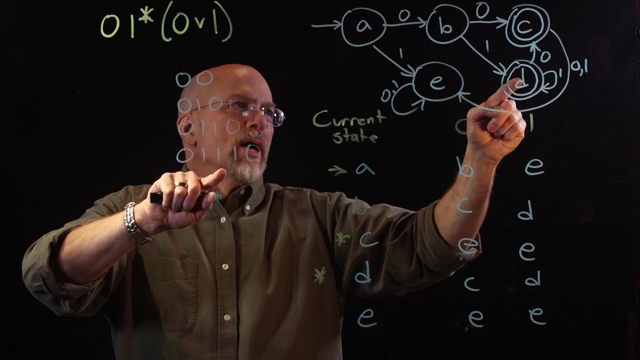 that was an element of the regular set for this regular expression. So we have zero, zero. We go to C. I have zero, one zero. That takes me to C. I've got a zero, one, one zero, And then I've got zero, one, one, one zero. And so all of those things take me to. 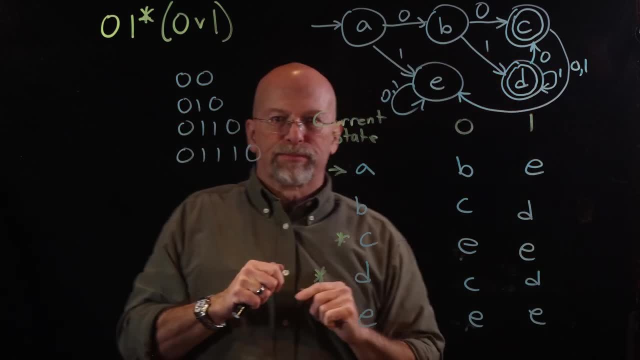 this one right here takes me to C. Now, if I get another zero, I've got zero. one one, one zero. If I get another zero here, that's going to take me to the non-accepting state of state E. 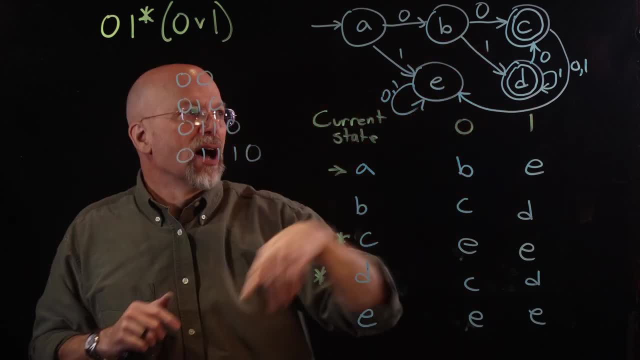 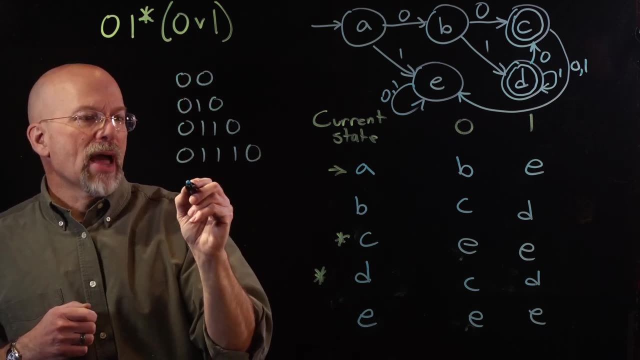 If I get a one, same thing happens: I come, I fall out of the accepting state. Now, what about the other way? What about if we end in a one instead of ending in a zero? Well, that was, let's see, zero one, zero one one, zero, one, one, one, zero, one, one one. 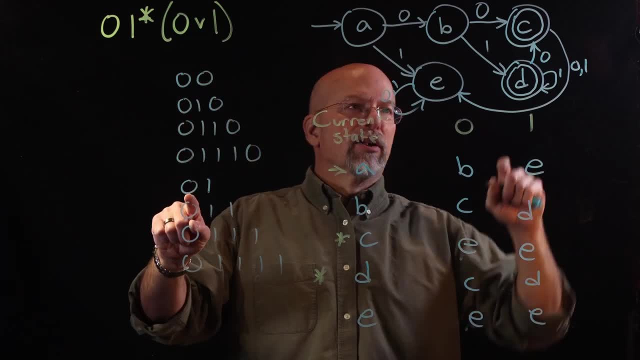 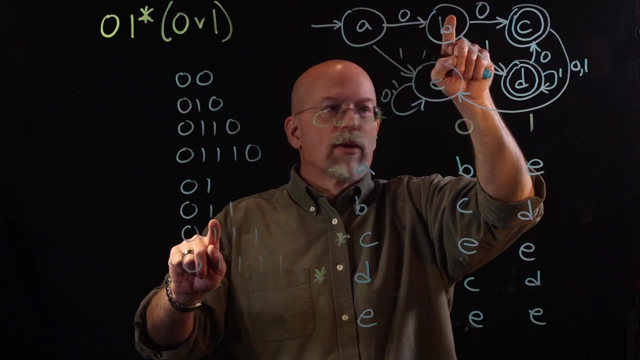 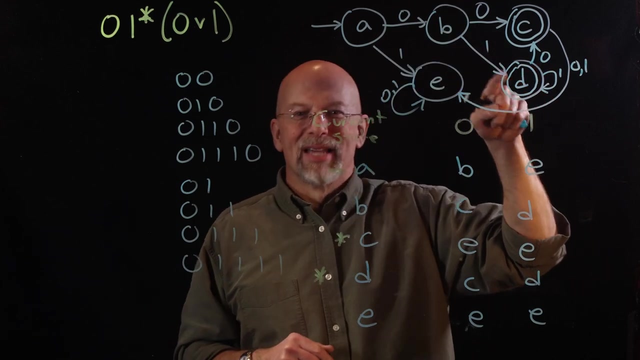 and so forth. So what you're looking at here is a zero, followed by a one. I'm in accepting state Zero, followed by a one, followed by another one. I'm in the accepting state Zero, followed by a one, followed by a lot of ones. I stay in the accepting state D, So this one really is the accepting state. 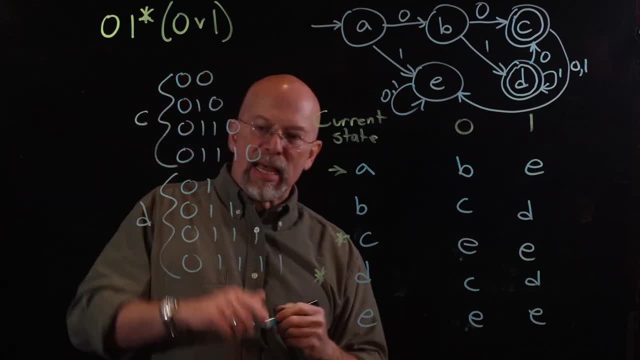 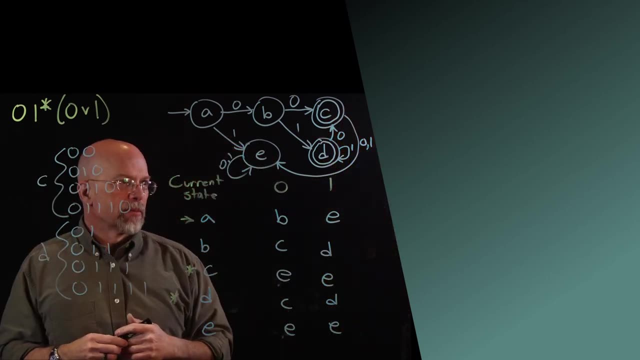 C. This one really ends in the accepting state D. If I get a zero after I'm in D, I go over to C. If I get anything else, then I'm, then I fall out. So this does look like an appropriate. 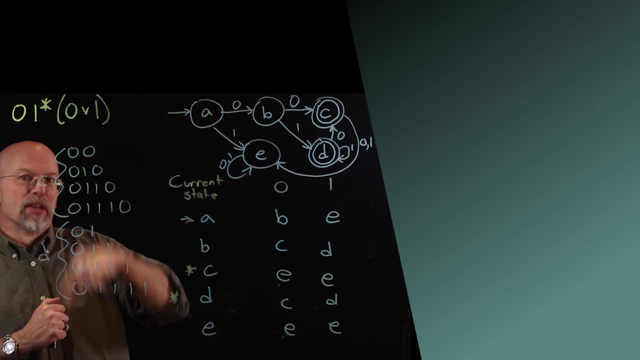 an appropriate determinant finite automata for the non-deterministic one that we started out with.